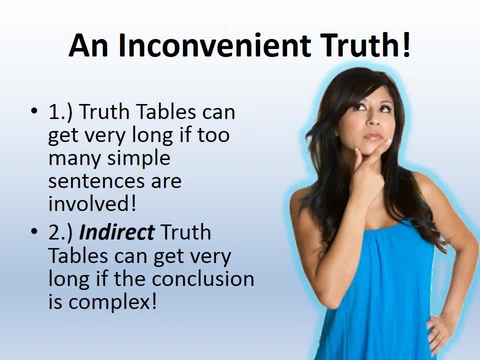 Now, what we've said about truth tables is that they have an inconvenient feature: that they can get very long if there's too many simple sentences being involved, And indirect truth tables can get very long and are hardly able to be done if the conclusion is too complex. 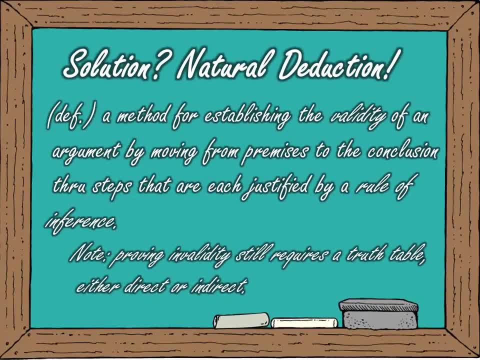 We needed a more convenient and powerful system. The solution we came up with was a natural deduction system, which is a system of establishing validity in a propositional argument by moving from premises to conclusions through intermediate steps. The key thing is that these steps, that 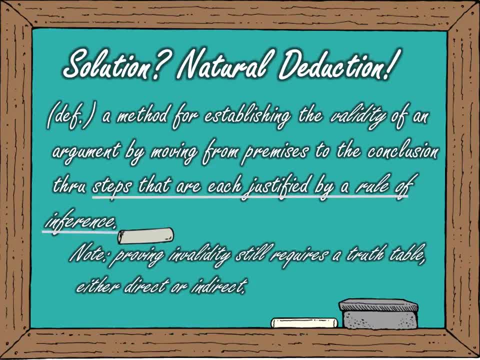 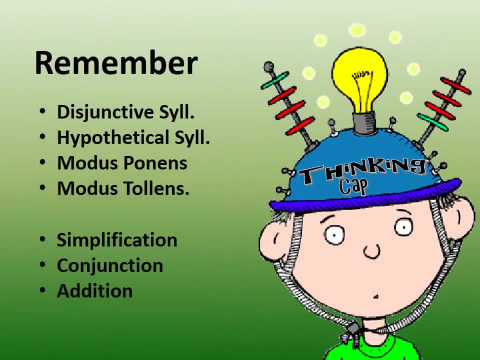 we make in the argument have to be justified by rules of inference. How to prove invalidity? We still need a truth table for that. I prefer the indirect truth table method. Now remember we've already studied seven rules of inference so far. I hope you've committed. 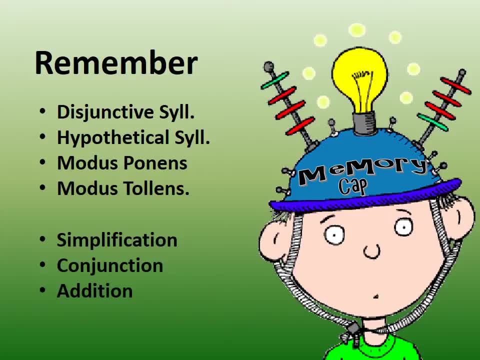 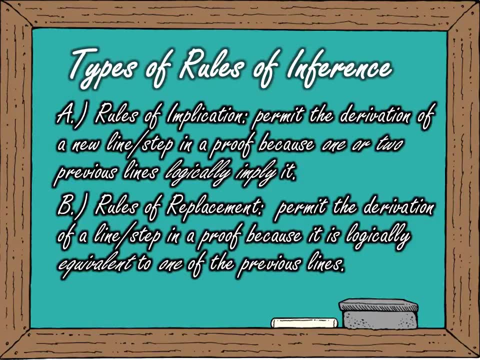 these to memory. There's no other way to handle them, But four were kind of difficult and three were extremely simple and very intuitive. Now these rules of inference still hold. We studied rules of implication in the last lesson. This time we're going to move forward. 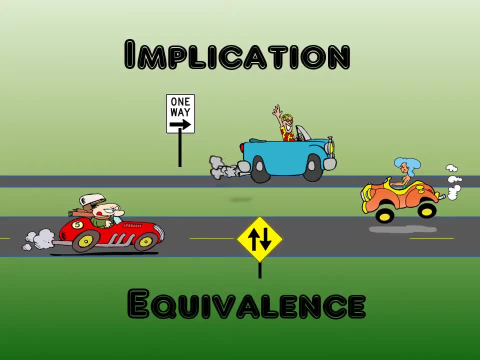 Remember, implication is a one-way street. Equivalence is kind of like a two-way street. For example, in the last lesson I said that the rules of inference are one way street. Equivalence is kind of like a two-way street. For example, in the last lesson I said that the rules of inference are one way street. Equivalence is kind of like a two-way street. For example, in the last lesson I said that the rules of inference are one way street. For example, in the last lesson I said that the rules of inference are one-way street. 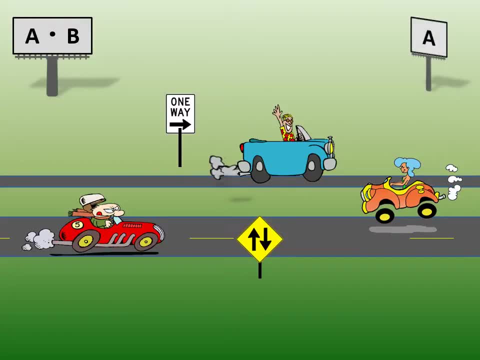 It doesn't go vice versa. A does not imply both A and B. However, by way of contract, A and B implies the proposition B and A, and vice versa. that sort of move is an equivalence Thing goes for things like A just being equivalent to B, and 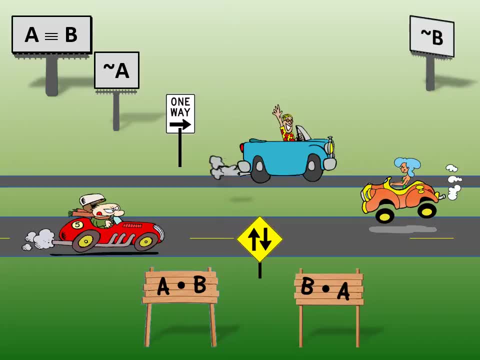 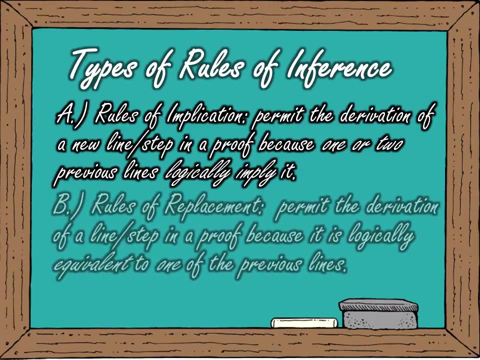 tilde A. Those two propositions combined imply tilde B. but you can't move from tilde B- the claim that tilde A- or to the claim that A is equivalent to B. It's not a two-way street. So in this lesson we're going to start studying rules of replacement, the equivalence claims. 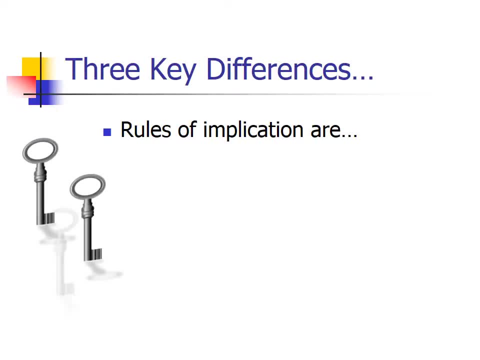 The difference is: the rules of implication are derivations of a line from one or two emphasis on or two previous lines in a proof. They are valid argument forms, like hypothetical syllogism and modus ponens, and they are applicable only to entire lines in a proof. 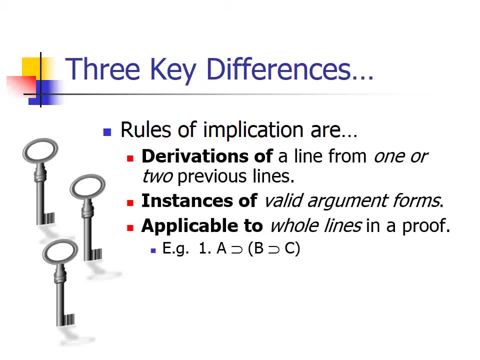 What I mean by that is, if you have a claim like A implies that B implies C, you can't take B and take a part of premise one and say I'm going to move to C by modus ponens. That is an incorrect move. You have to apply modus ponens to the entire proposition of 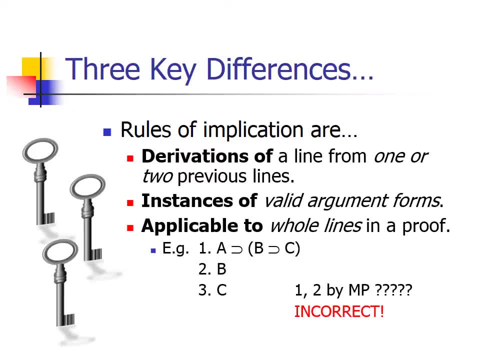 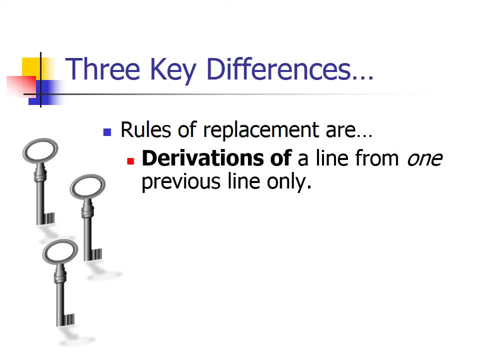 number one, and just not. you can't just take a part of the proposition and use it to do modus ponens. That's invalid. Now, the rules of replacement, by way of contrast, are derivations from only one previous line, because the line you derive is logically equivalent to the line you derived. 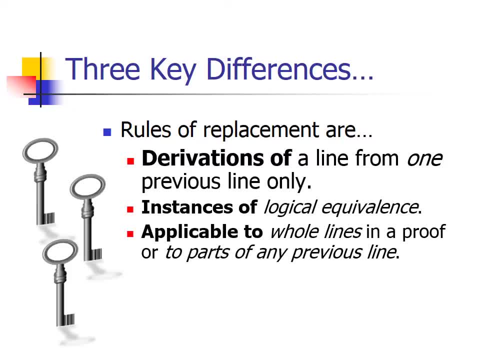 from And they are applicable to entire lines in a proof or important difference to parts of a line. So you could take something like A implies B and move to the claim by double negation that A implies tilde tilde B, Tilde tilde B and B say about the same thing, So you can apply these rules. we're going to. 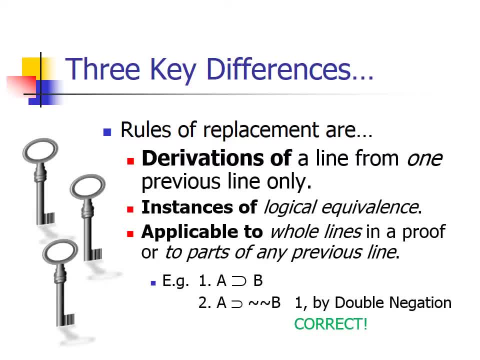 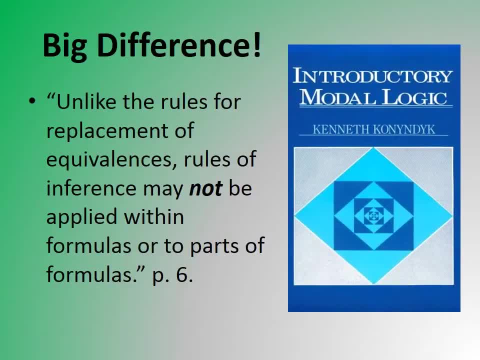 study today to parts of lines in a proof. Big difference, As Kenneth Conan Dyke puts it in his Introductory Modal Logic book: unlike the rules of replacement of equivalences- that's the stuff we're going to study today- he says rules of inference. 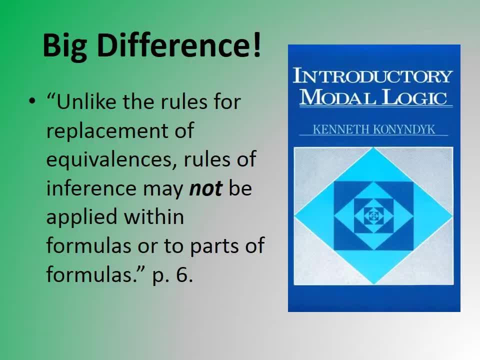 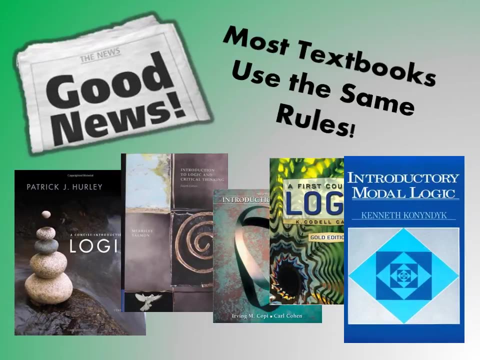 the stuff we studied last time may not be applied within formulas or to parts of formulas. They cannot be applied to parts of premises or to parts of formulas. The rules we studied previously have to apply to lines as a whole. Now the good news is most textbooks use the same rules, and this distinction between the 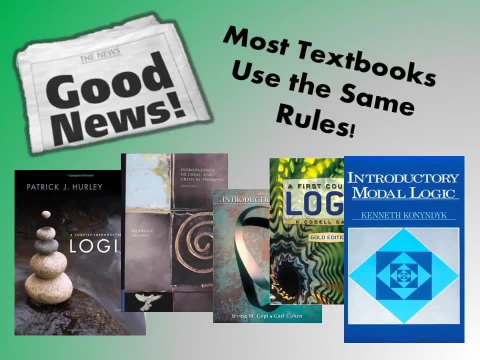 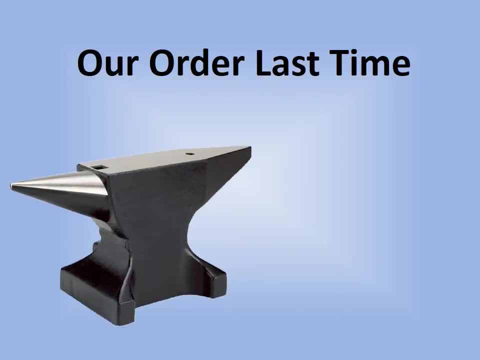 rules of replacement and the rules of equivalence is going to hold throughout any textbook that you study in a college level course. So let's get underway. Well, last time when we studied our rules, we took it in this order. We said we're going to study the hard stuff first and then we'll go ahead and move to some simpler rules, like 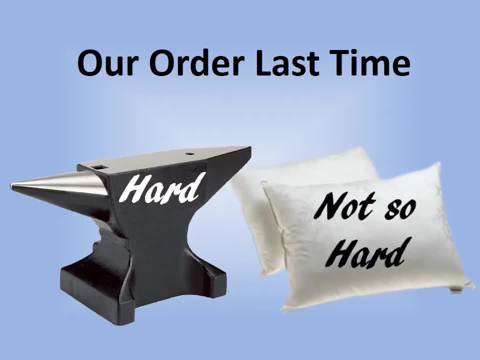 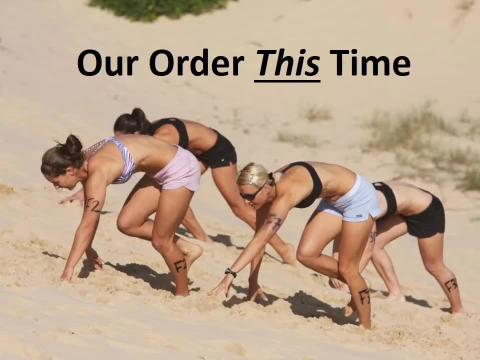 simplification and things of that nature. This time we're going to do things differently. This time it's going to be an uphill battle When we study rules of equivalence. I'm going to give you the easy stuff first, the stuff that's intuitive, and then we'll 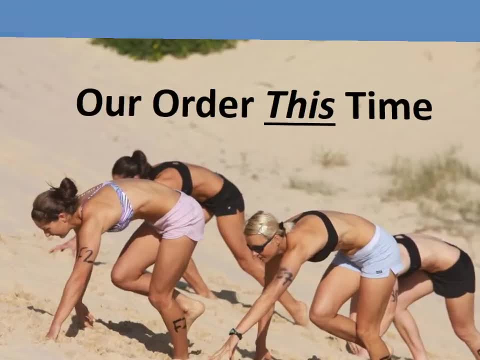 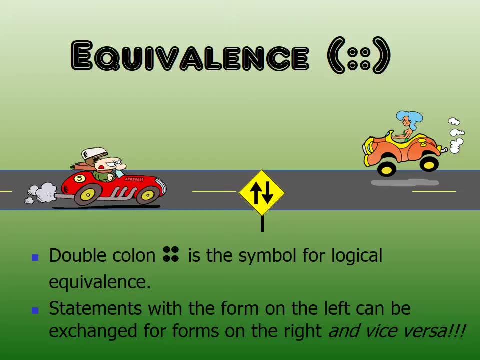 work up to the difficult rules of equivalence later on. Now, when we talk about equivalences, I'm going to use a double colon as the symbol for logical equivalence. What that means is that stuff on the left can be exchanged for stuff on the right and vice versa, That basically, they say logically the exact same thing, Two way. 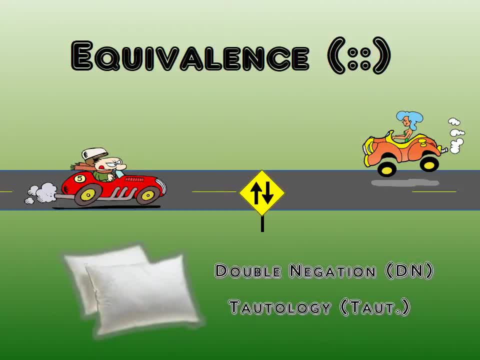 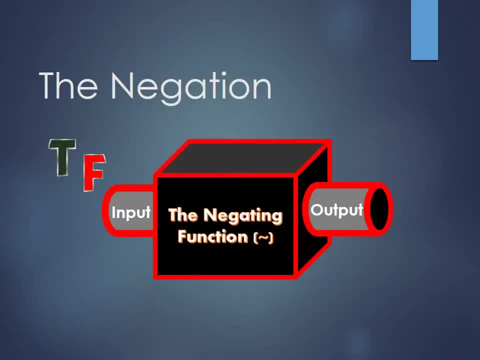 street The first two really easy rules of equivalence, Double negation and tautology, and get those under our belts. Now, when we talk about the truth function for the negation, what we said is it's basically the flip flop function. It just takes whatever truth value you put in of a proposition and 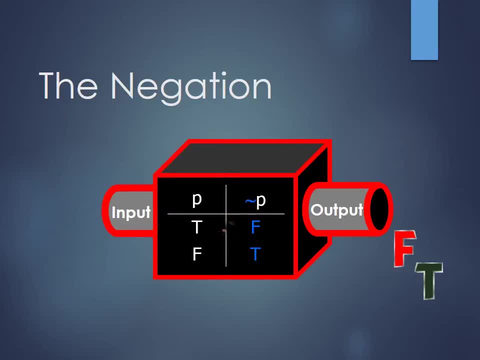 it spits out the opposite value And that's because of the truth table for the negation. It's truth, functional definition, But the negation doubled. then If we take these truth formulas and run them through a second time, you should return back to your original value. 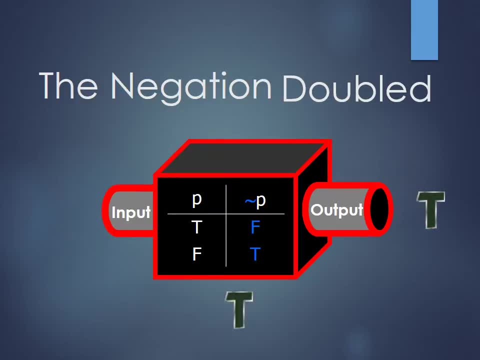 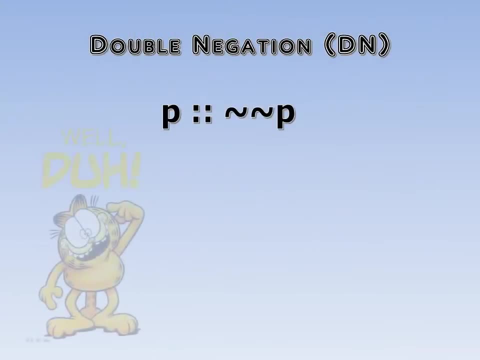 right, That makes perfectly good sense. And that just means that, basically, a double negative is equal to the original value of the proposition. So, basically, P is equivalent to tilde, tilde P and vice versa. Makes perfect sense, right? So, even when you're dealing with complex propositions, 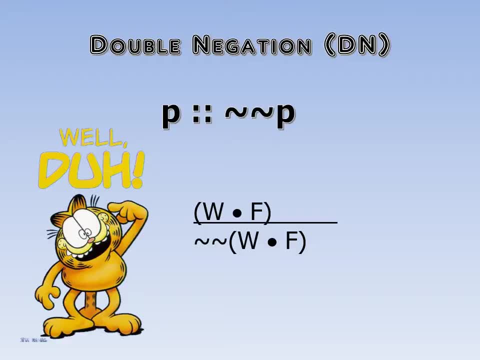 like W and F, you can double negate that entire conjunction and you've said the exact same thing thing. Of course, if you take a simple proposition like U, you can move from the double negation straight down to the unnegated version and vice versa And look at a proposition as long 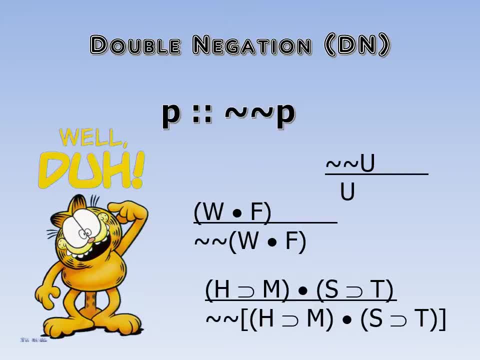 as the one I gave you at the bottom. Make sure you put brackets around the entire thing before you add double negatives. As long as you do that, you've ended up with an equivalence. You can move from one to the other and, importantly, you could go vice versa, But also you can. 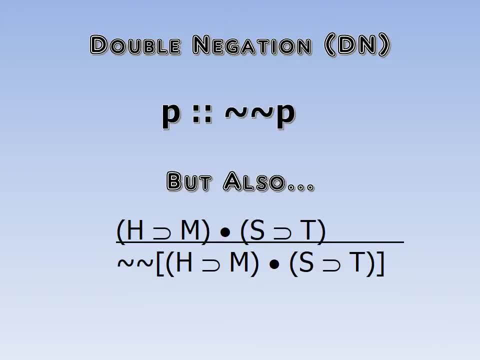 apply these sorts of equivalences to parts of proofs or parts of lines. I should say: What if, instead, I wanted to take the latter part of the original premise- S implies T and double negate that. That's perfectly acceptable. Or if I wanted to take some simple proposition. 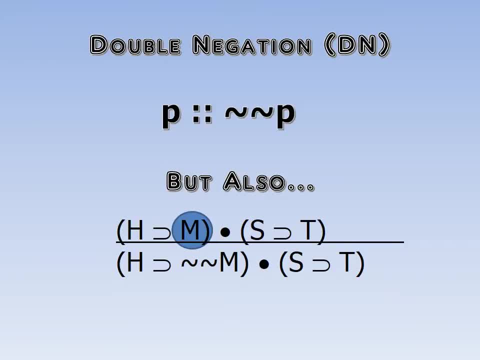 embedded deeply in the long, complex one. I'll take M and double negate that. That's okay, because tilde, tilde, M says the exact same thing as M. Or if I wanted to take a simple argument, I could take S and double negate that, or vice versa. Not a problem, They're. 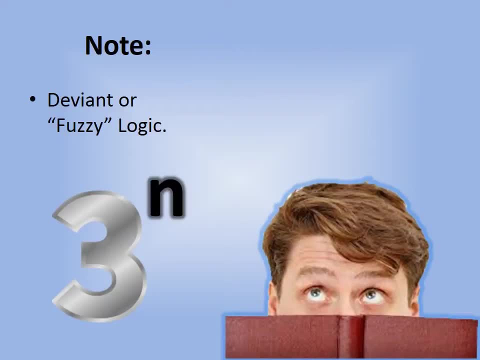 equivalent. Now there are forms of logic that involve three truth values. If there was a truth value that was neither true or false, well then our double negation function would not work. But we're doing classical logic, the traditional forms of logic, and we recognize two truth: 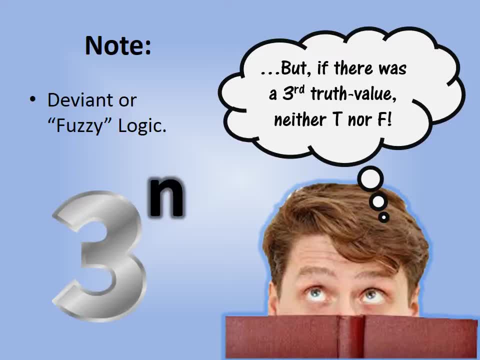 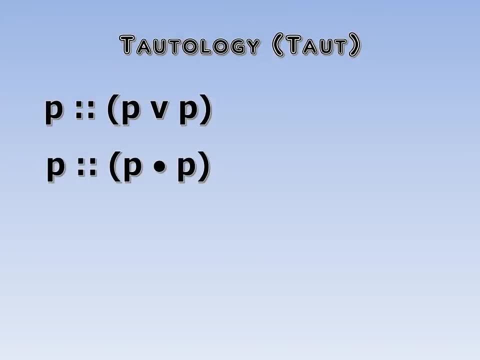 values, And true is the opposite of F and vice versa. no middle ground. That's why this negation function works the way it does. Let's talk about tautology. That's another simple one: P is equivalent to P or P, And. 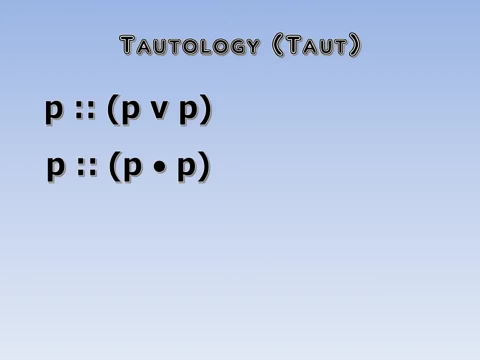 the same thing happens with the dot. P is the same thing as P and P. Now we already have studied something like these rules. We had a rule called addition which said that if you started with a proposition P, you could wedge it to anything. The tautology rule says: 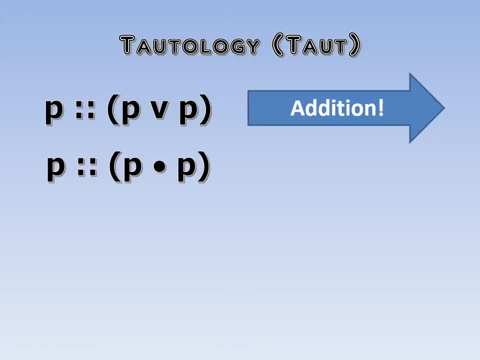 if you have the exact same proposition on each side of the wedge, you can eliminate one side. That's something new. And we did have a rule that said if you have P and P, you could simplify down to P. That was a rule for the conjunction, But now this rule says: if this proposition on each side 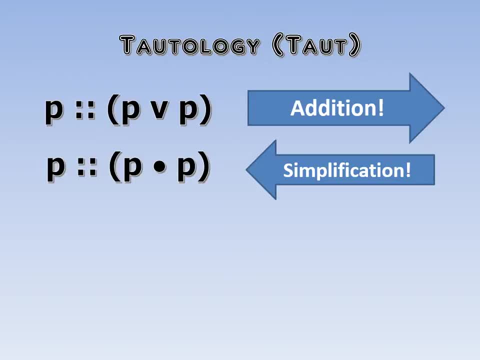 of the dot is the exact same proposition, then it becomes a two-way street. So very often this rule is just a technical help. It may seem tautologous, as the name implies, But for example, you're not going to get through an argument that says A or 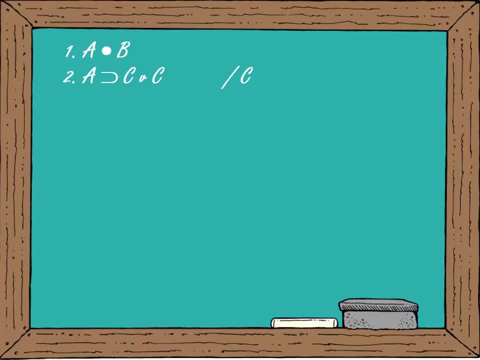 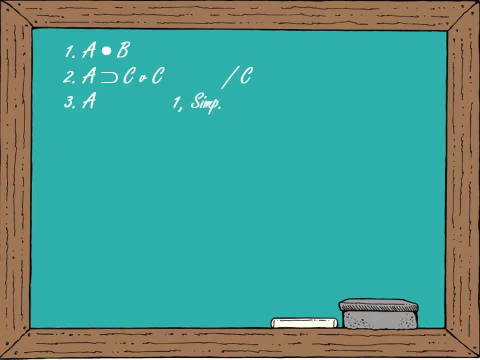 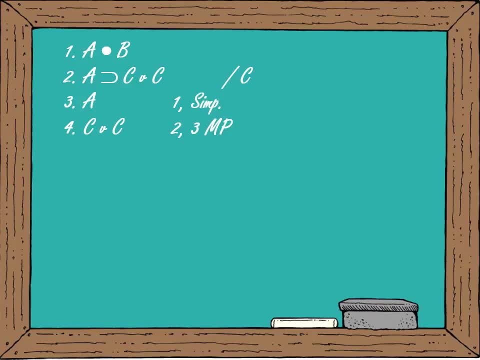 And so, for example, if it's not A, then it is A sub A, sub A, sub C, sub A sub B. And now notice that this is a very complicated rule. So let's look at this, Let's look at this, Let's take a look at this. 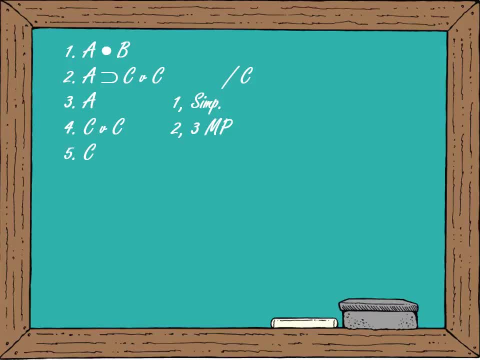 So this is a point ofтя: you can reach A by simplification on one and by modus ponens. then you can reach C or C, That's not a problem. But then to get to the conclusion that's C, you've got to have something that allows you. 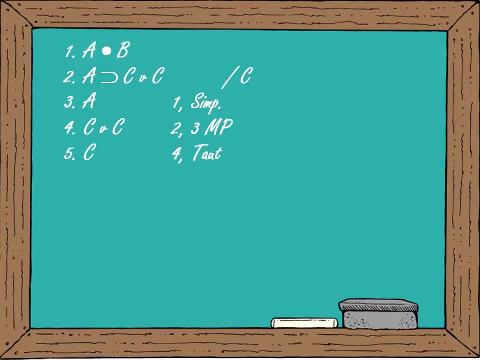 to eliminate the wedge, and that only happens when both sides of the wedge say exactly the same thing. Then the move is tautologous. Or, for example, P implies that, not Q and Q. Well, if Q is true, then does that mean P is false? Well, it seems like we should be able to. 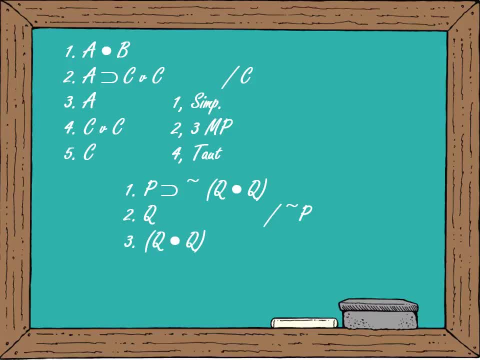 reach that by modus tollens, but only if we have a rule that lets us move from the claim that Q to Q dot Q Tautology will. let us do that Then by double negation. we have the negation of the consequent in premise one. Once we have 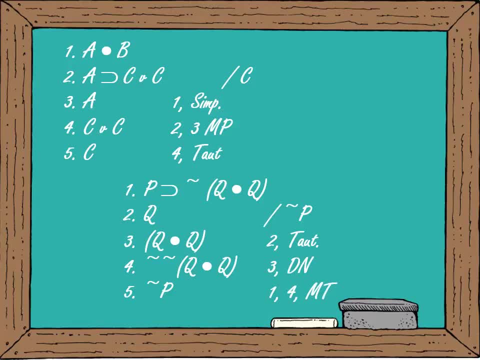 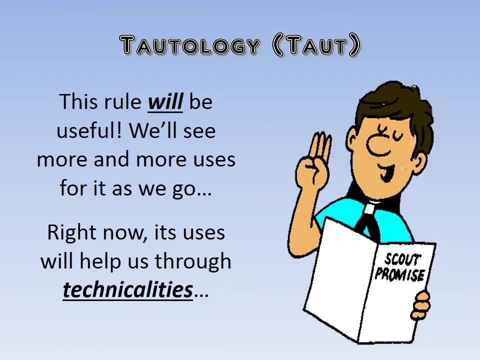 that we can move to tilde P by modus tollens. See how it works Now. this rule may seem to be just a technicality, but it will be useful and we'll get more and more uses as we go on. 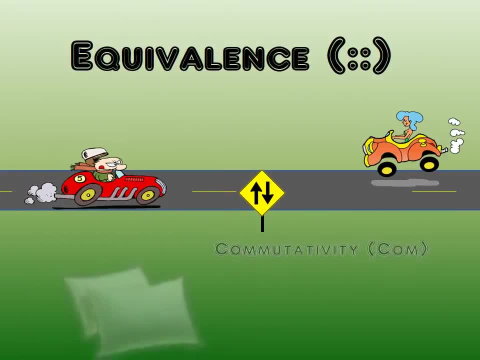 Scout's honor. Well, let's talk about more equivalences. How about commutativity and associativity? Very soft, simple rules. As the name implies, commutativity involves some sort of commuting. If you've ever been a commuter, you know that means. 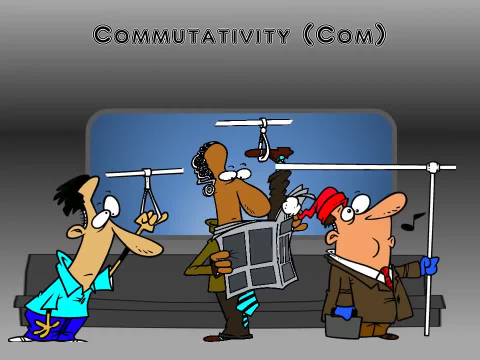 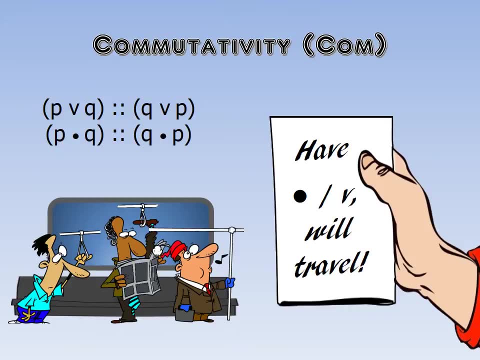 traveling. We're going to let propositions travel a bit. That's a good mnemonic device for remembering this rule. Commutativity means if you have a dot or a wedge, you can let the propositions travel. P, wedge, Q is just Q, wedge P, P, dot, Q means 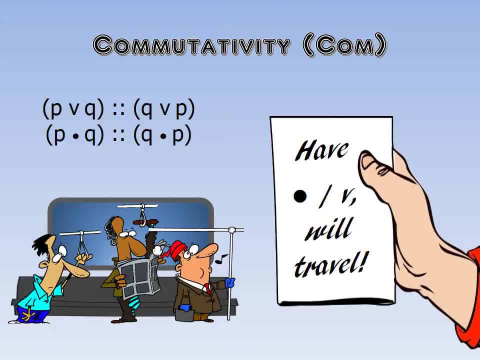 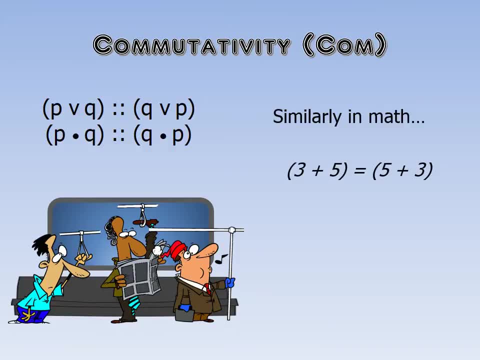 Q, dot, P Around the wedge and the dot propositions, however complex, can do some traveling. In fact, it's similar to a situation in math where you can flip-flop around the addition symbol 3 and 5 means 5 and 3.. 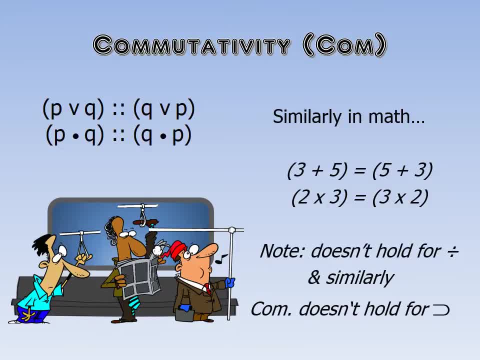 2 times 3 is 3 and 2.. There are other connectives, just like there are things like division in which it doesn't hold. For example, commutativity won't hold for the horseshoe, just the wedge and the dot. Remember that. 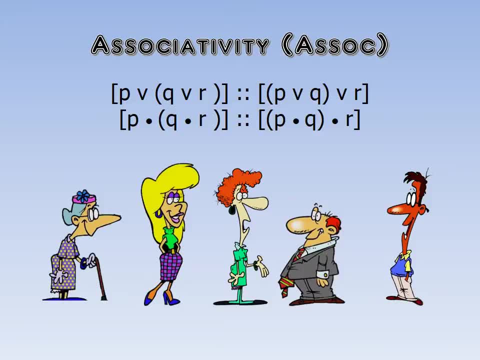 Associativity. Well, here's another mnemonic device for you. If you have three propositions involved and all the propositions are linked up with like a wedge or a dot, well then you can start moving the parentheses within them so that propositions associate with other propositions differently. 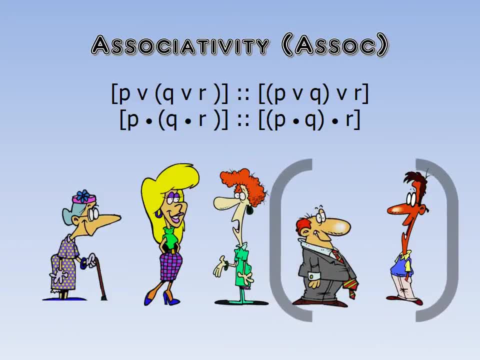 Kind of like you can associate with some people or you may choose to associate with others- It's your choice- Or vice versa. When you can move the brackets or parentheses around in this fashion, that's called associativity, Kind of like associations you keep with people. Now. 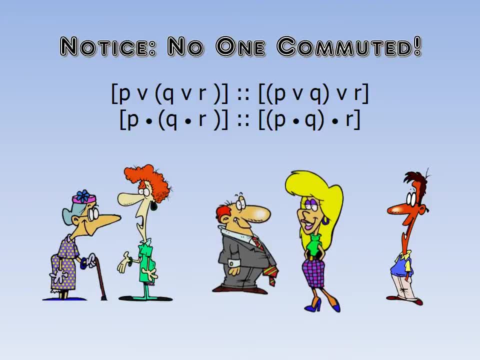 notice. no one commuted, Nobody traveled from spot to spot here. The P's, Q's and R's in our propositions similarly Did not move. This is not the same rule as commutativity. It's a rule for moving parentheses and brackets, And the same. 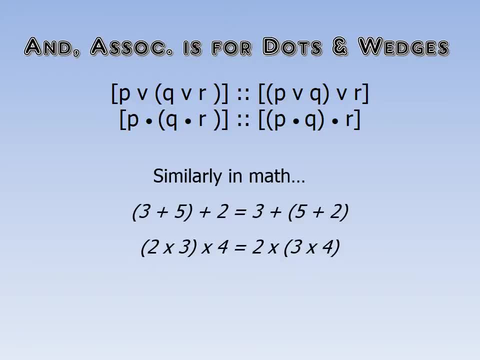 thing holds for associativity as commutativity, namely that it only applies to dots and wedges. For example, in mathematics, 3 plus 5 plus 2, as long as the plus symbol is moved throughout, you can move the parentheses around. That's the same as 3 plus 2, 5. 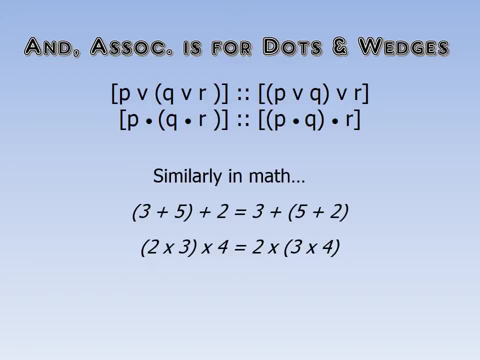 plus 2, with the brackets or parentheses moved slightly to the right. Same thing holds with multiplication, And again it doesn't hold for the division symbol in math. And similarly our rule for associativity does not hold for every single connective either. 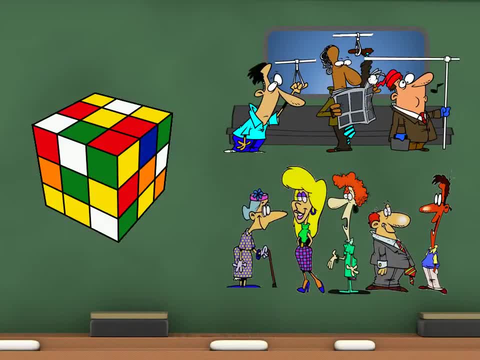 It doesn't hold for the horseshoe. So when you have this sort of rule in your pocket, you can start moving propositions into place in order to get your proofs to work. That's really what these two rules help us out with. Let's do a little. 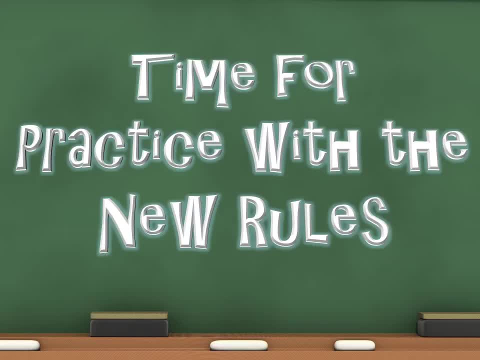 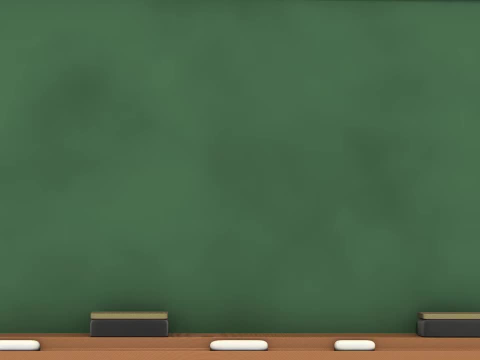 practice with these new rules that we've just gotten under our belts, so we can see how they help us solve proofs that we could not have solved in a previous lesson. So how about this? one Suppose I have tilde j, gives me tilde k and a premise that says: 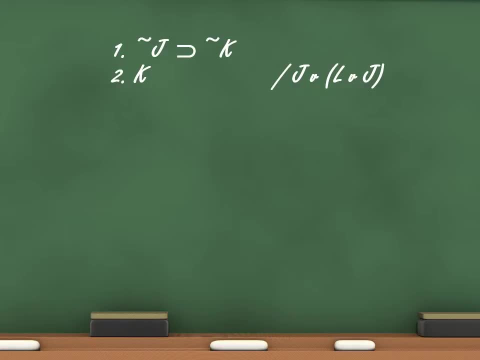 tilde k. Well, obviously I can do something with these two premises like modus tollens, and I should be able to get to a conclusion out of them, like j, very simply. But look at the long conclusion I have here: j wedges to, l wedge j. Well, after I get to. 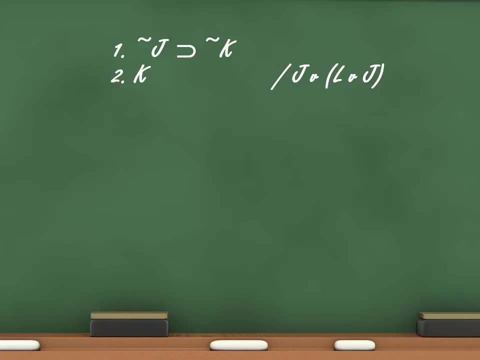 j. I should be able to get to something like that, but I'm going to need a lot of my new rules in order to get that long conclusion, So let's just use the obvious. My second premise is pretty much equivalent to double. 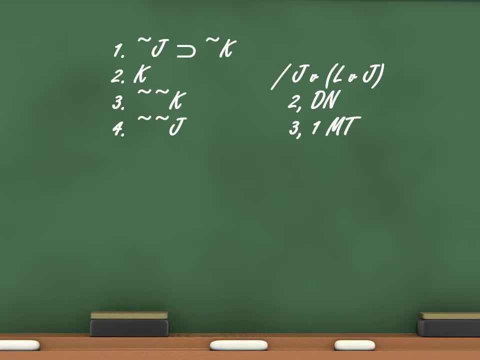 negation k and that's going to give me, by modus tollens, the tilde, tilde j. Now, where do I go from here? Double negation will help again. Look, I finally got my j. What do I do now? Well, what I'm going to do is I'm going to reach j or j by tautology. 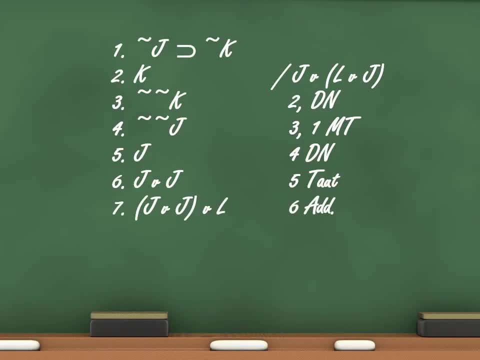 because my conclusion has a second j in it. Then I'm going to wedge that off to l, because rule addition says I can wedge off to anything I want, And after that I'm going to have to use associativity to move my parentheses down towards the right where I need them in. 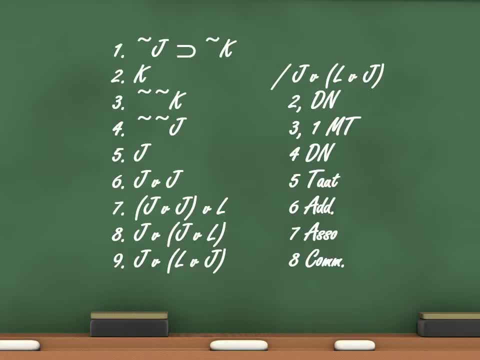 my conclusion. By commutivity I get to my conclusion. I can just move j or l into each other's spot. They do a little traveling or commuting around the wedge. My proof is done. For example, here's a more well, rather a more complicated example: p, dot, q, dot, p, and. 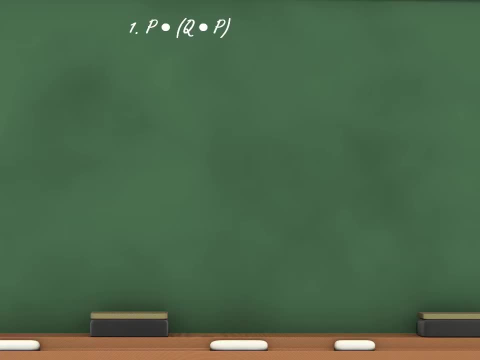 with some brackets thrown in there. This asserts both q and p, So I'm going to have to use associativity to move my parentheses down towards the right, but the propositions are locked up pretty tight. I need q and p to work with premise. 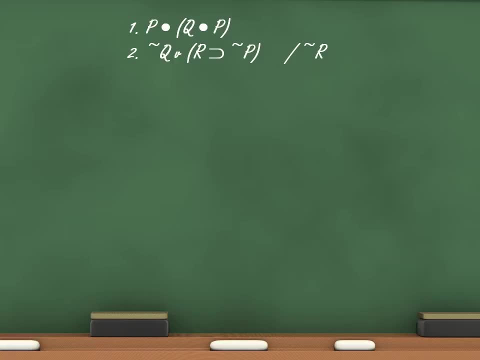 2. If it says that q is false, which of course premise 1 says it's not, then r implies tilde p, But of course premise 1 says that tilde p can't be the case. Can I get to tilde r? 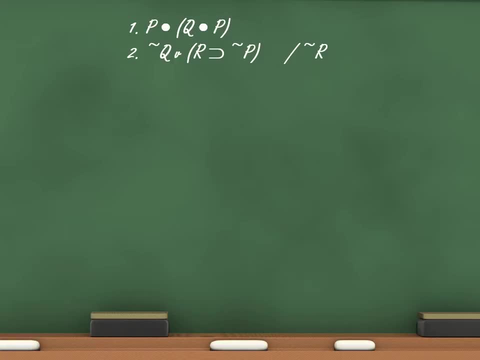 I need to start unlocking my p's and q's in order to work with premise 2.. So I'm going to start by moving the parentheses in premise 1 by associativity and then flip-flopping the positions of q and p. Why do that? 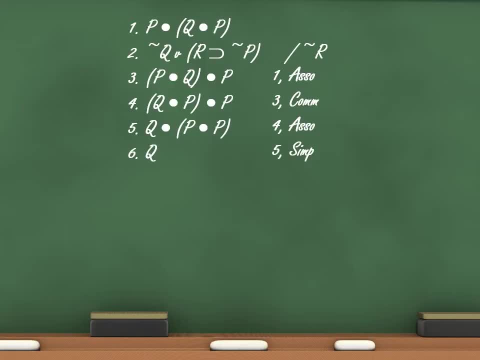 I can move the parentheses back by associativity once again and unlock q. I need q so that I can double negate it and use premise 2 by disjunctive syllogism to get to the horseshoe claim. Now, once I have that horseshoe claim, I look back at premise 1.. I have a rule called 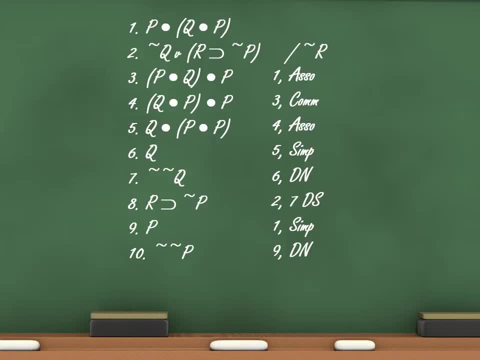 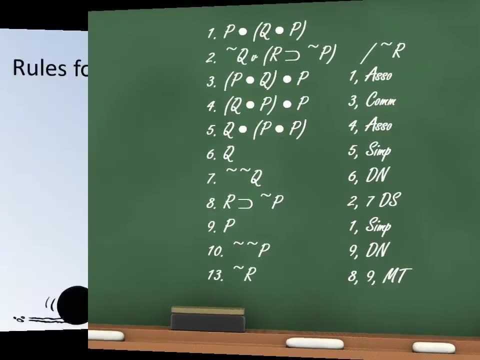 simplification that allows me to get straight to p. Once I get p, I can double negate it. do modus tollens on premise number 8, and then I'm home. free Subtitles by the Amaraorg community. Page 1 of 1. 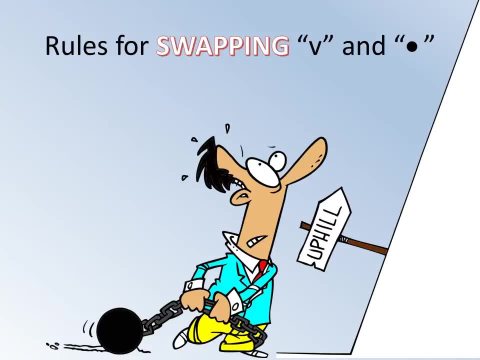 So associativity and commutivity are very helpful in getting back through these sorts of proofs. but notice, we never swapped out a wedge claim for a dot claim or a dot claim for a wedge claim. As we struggle uphill towards more complex rules we're going to discuss. 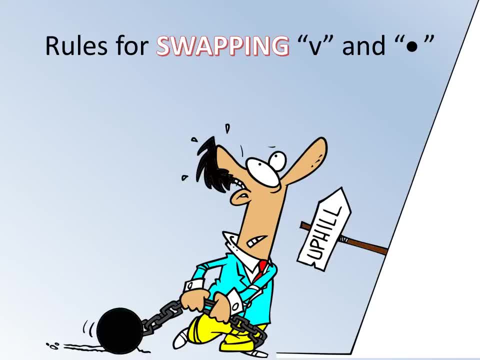 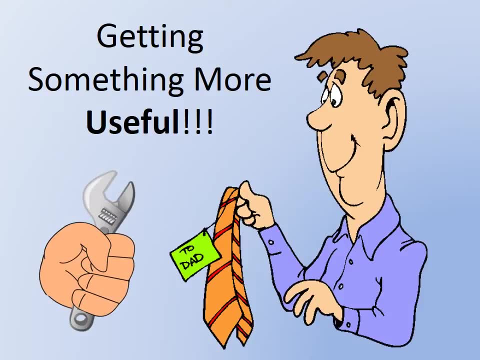 rules that allow us to exchange one type of these claims: a disjunction for a conjunction or vice versa. Why do that? Well, sometimes you just need something that's more useful in your proofs. For example, dot claims tend to be a lot more help in a proof than wedge. 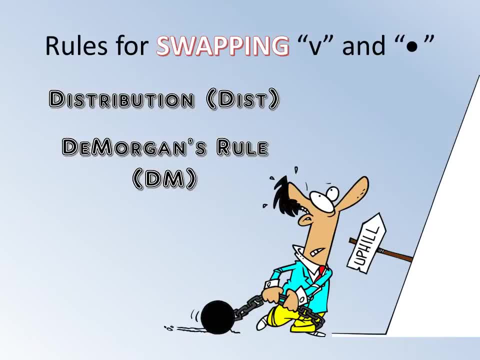 claims, because dot claims give you more information. So our rules for swapping out one of these operators for the other are the rules of distribution and De Morgan's rule. As we struggle uphill, let's try and wrestle with these more complicated rules for logical operators. 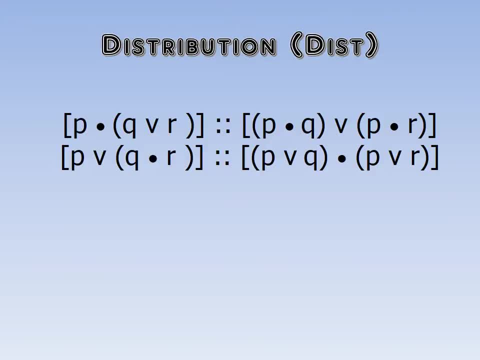 Now the rule of distribution. there's no getting around it. This is a complicated rule. As you try to memorize these principles, I want you to notice two things. Number one: the key thing is that the main operator changes as you move from left to right and vice versa. 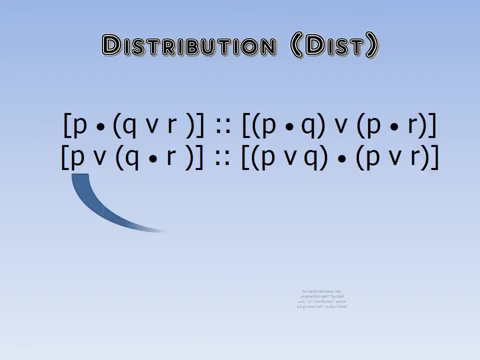 And that's the most helpful feature of this rule. And secondly, it's called distribution. because of the move from the left to the right, P gets distributed in the way that it's forced to associate with the Q and R respectively, hence the term. There's no getting around. 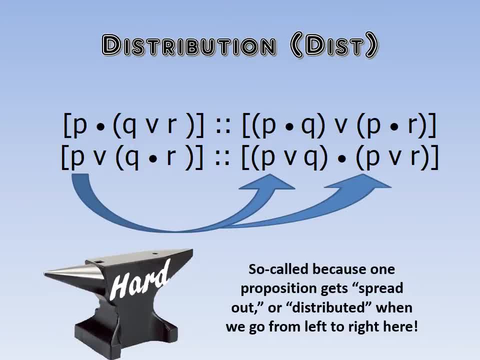 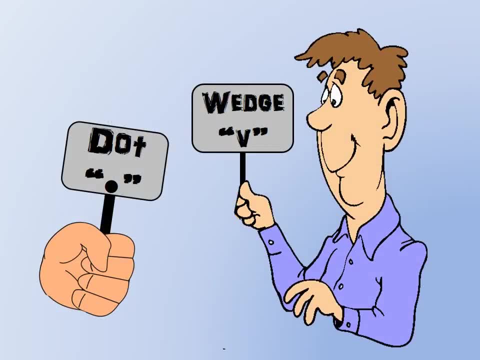 it. This is a hard rule and you're going to have to spend some time committing it to memory and even more time learning how to use it, But it is very helpful for getting some. I find it especially helpful when I exchange a wedge claim which doesn't have a whole 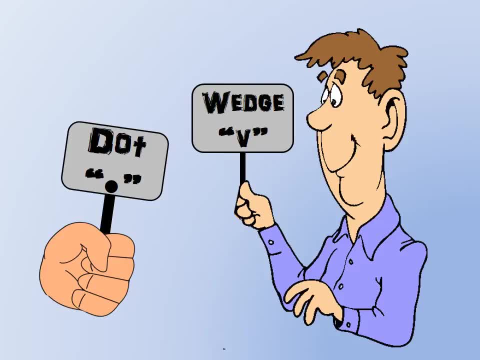 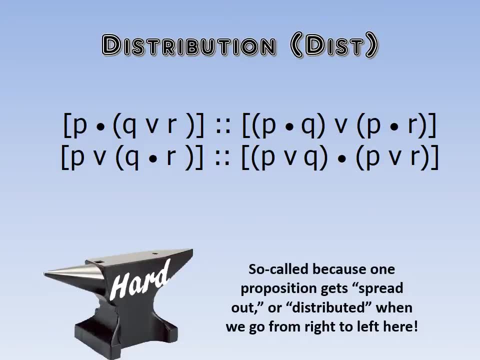 lot of information in it for a dot claim. The wedge claim is a dot claim which I can simplify to one of the other conjuncts And that's very helpful in a proof. Another interesting feature of this particular rule is that, unlike the rules that we studied, 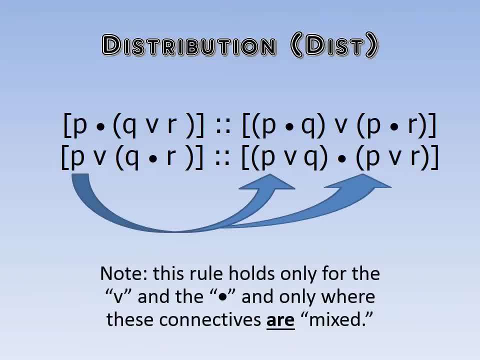 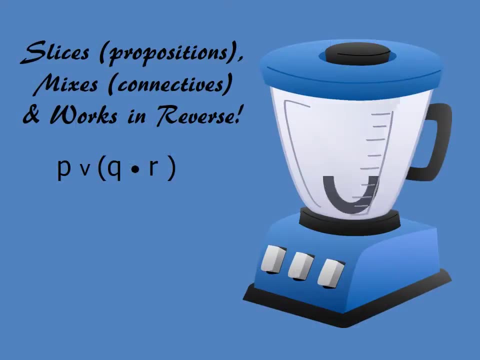 previously. it's one of those rules where we also have a situation where the wedge claims and dot claims are mixed. Associativity and commutivity just involved one of these operators, wedges or dots respectively, throughout the entire proposition. I don't know why, but 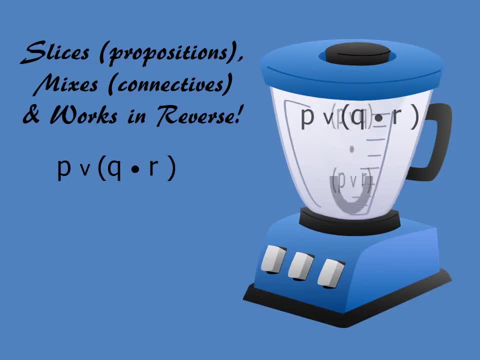 this always helps me Remember the rule. It slices, dices, mixes and matches. It slices up the proposition P and distributes it and it mixes up the connectives and it even works in reverse. I don't know why, but that helps me. 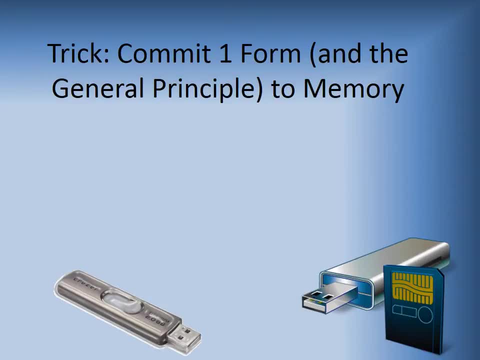 remember it. Another way to remember this rule is just to commit the first form of it, that the implication goes one way. Commit that principle to memory and then the other principles. well, the other versions follow the same general principle. Use these sorts of tricks to help. 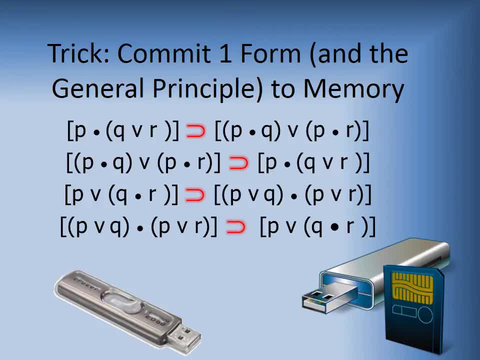 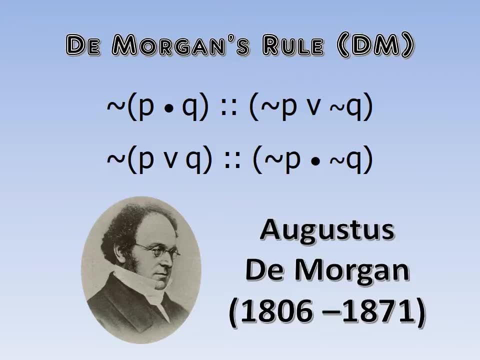 get your mind around the distribution rule. It can be very helpful. Well, in a previous lecture we already discussed De Morgan's rule, so hopefully you're already familiar with that. It's named after Augustus De Morgan, the 19th century logician who discovered 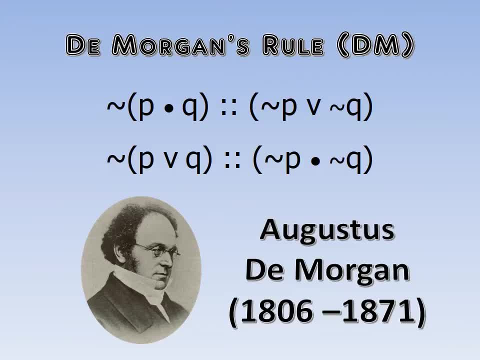 that tildes could distribute in a unique way that allowed you to change wedge claims to dot claims or dot claims to wedge claims. Again, you're going to have to do some memorization here, but the principles should be pretty clear. Now the reason why this works after you've. 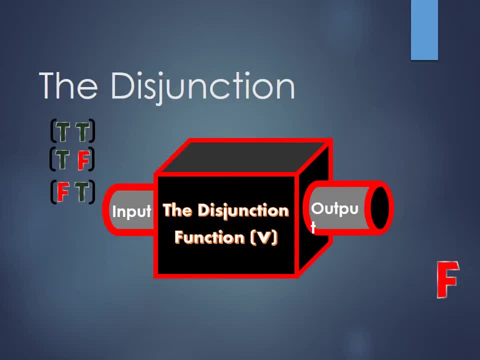 memorized those two principles is because it allows you to change wedge claims to dot claims, because the disjunction function is basically one that allows you to put in inputs of a certain sort and get out truths of a certain sort. It only gives you an f when you get f's for both. 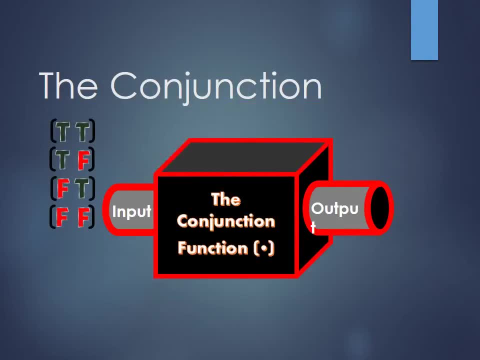 disjuncts the bottom end of this table. The conjunction function, by way of contrast, is only going to give you an f. well, it's going to give you an f on every occasion, except for the situation where you put, in truth, values t for both propositions. That's just the. 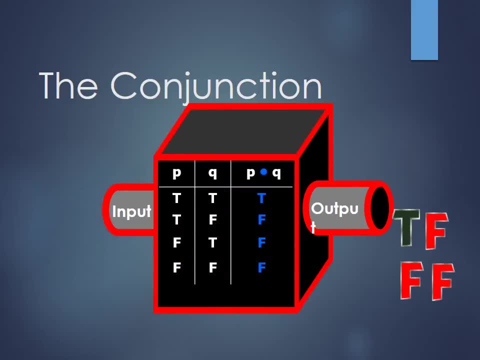 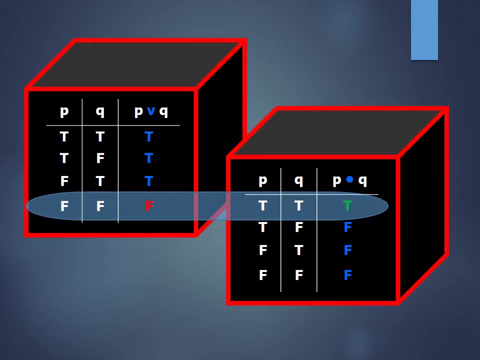 way our table worked. Now take a look at these two tables. What you notice is the only time that you get an f is pretty much parallel to the only time you get a t for the conjunction. It's a unique parallel here that allows De Morgan's rule to work the way. 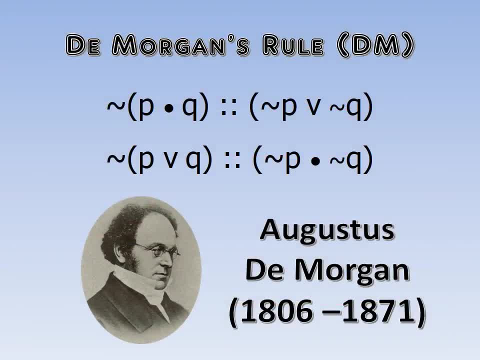 it does. So here's a little mnemonic device to remind you how to distribute the tildes across conjunctions or wedges appropriately. What you do with De Morgan's rule is you get a different main connective when you move the negation. So you get a different main connective when you move the. 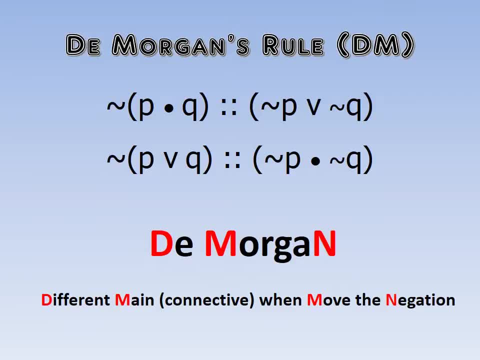 negation. That's the way you work it. Hopefully you guys can see how negations distribute or undistribute depending on how you go left to right or right to left, And the main issue here is you get a different main operator and when you do that, that is very helpful in doing your proofs. 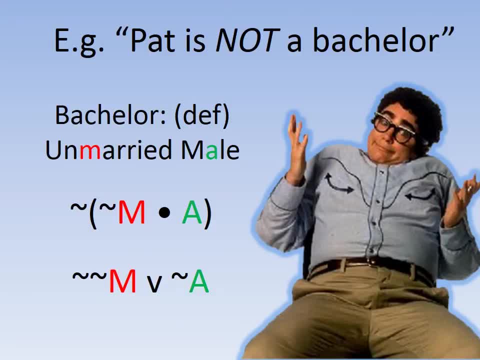 Well, here's a fun little example from Saturday Night Live to help you get your mind around De Morgan's rule and what it can and can't prove. Suppose somebody says that Pat, the SNL character known for his or her androgyny, is not a bachelor: He's not a bachelor. He's not a bachelor. He's not. 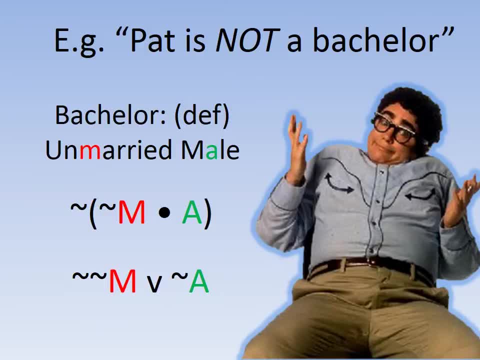 a bachelor. Well, does that little bit of information help you solve the mystery as to whether Pat is male or female? A bachelor is, by definition, a, not married male. So basically, if Pat is not a bachelor, you get tilde parentheses, tilde m dot a. So what does that tell us? by De? 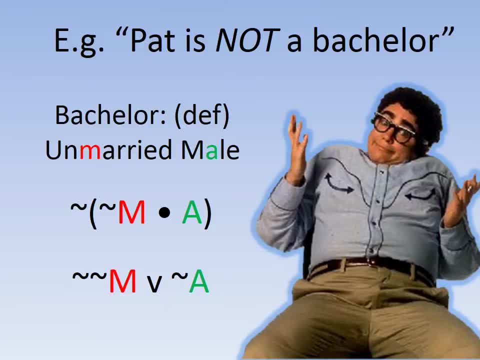 Morgan's rule. Well, I shift the tilde in across the tilde m and to the tilde a and I change the main connective to a wedge. So what we find out is that either Pat is married or De Morgan is married. 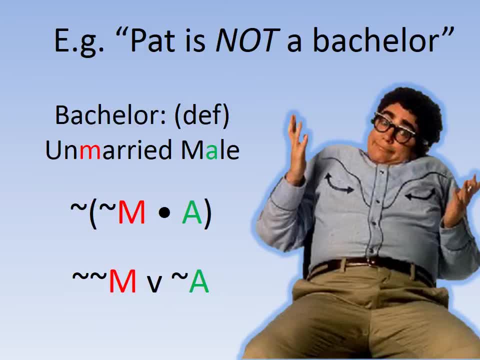 Or not a male. Does that tell you enough? Well, unfortunately no, it doesn't, unless you know the marital status of Pat. So I guess we can't solve a whole every mystery with De Morgan's rule, but it. 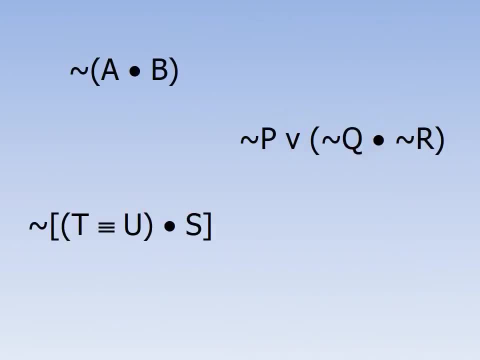 gets us a little closer in some cases. Just a little fun for you, Let's take a look at a few examples of how to use De Morgan's rule. How about the first up in your upper left? I'm going to use De Morgan's rule by first moving the tilde to the insides and changing the main operator. It's a. 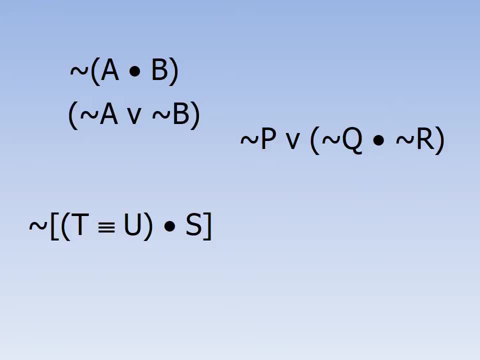 two-step process Now over in the next example. I'm going to use De Morgan's in this spot. First thing I'm going to do, I'll change the main operator and, secondly, move the tildes to the outside of. 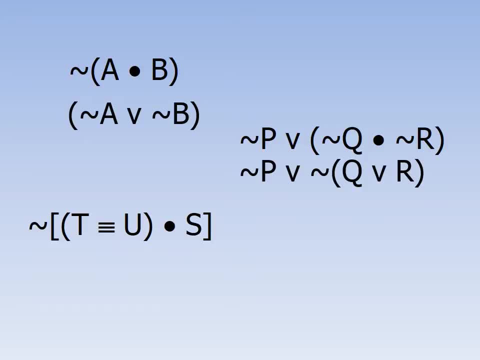 the parentheses. so it governs the operator that we just changed from a dot to a wedge, But I could have used well now I'm in a position to use De Morgan's in this position. Again, it's a two-step process. Change the main operator, move the tildes to the outside of a set of brackets. That way the 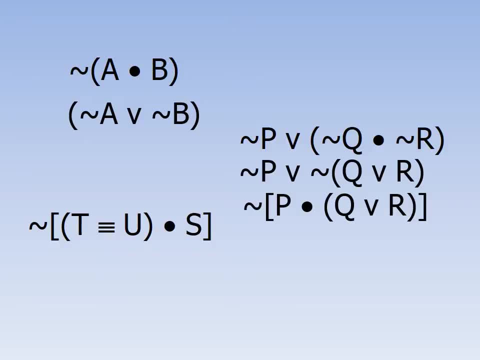 tilde once it's moved. it's going to be a two-step process, So I'm going to use De Morgan's in this situation. I'm going to go ahead and distribute the tilde to the inside, So I'm going to change the. 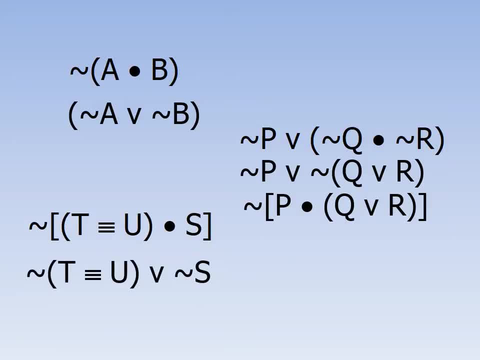 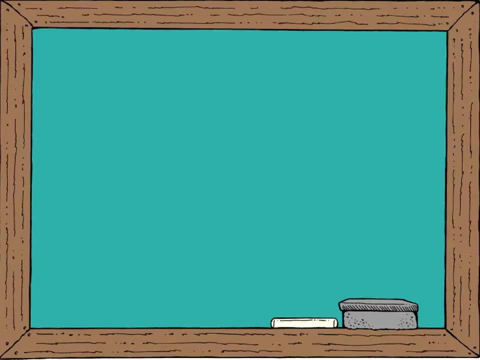 main operator and distribute the tilde- See Two-step process- every single time. Well, now that you know De Morgan's rule and distribution, let's find an example of a proof where you have to use both of these rules in order to get to the conclusion. In this premise we have a negation of the 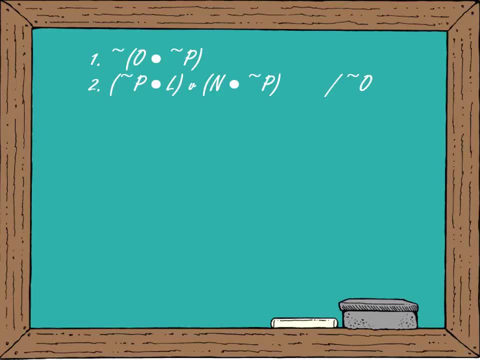 condition governing conjunction, And in this one you notice, curiously enough, that tilde p occurs twice. the second premise, That's a premise that we're going to use distribution on, We're going to try and reach the conclusion: tilde o, And I want you to pay attention to the fact that o is up there. 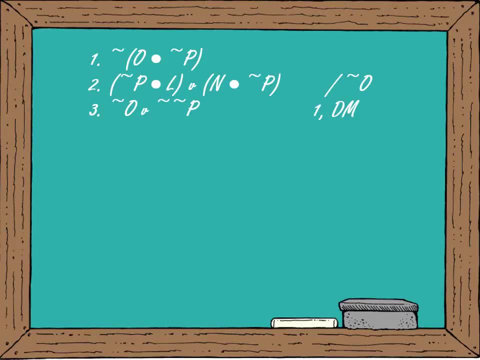 in premise number one. Well, first thing, I'm going to try and get o out into the open by using De Morgan's rule on premise number one. Now, notice, I'm set to get to my conclusion: tilde o. if only I. 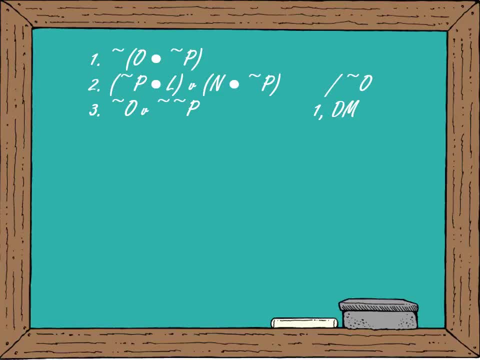 can do disjunctive syllogism of some type on premise number one. So I'm going to go ahead and look at premise three, or rather step three. So what I need to do is try and get to something like: 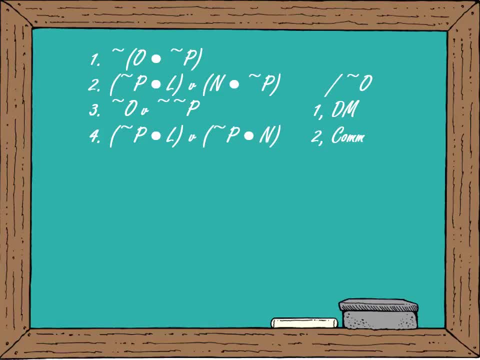 tilde p. Now tilde p is locked up there in premise two. I use commutation to put it in the right position, and distribution to get p outside of the parentheses and by itself. Then I can get tilde p by itself through simplification. Now I'm almost set to use my disjunctive syllogism. I just need to. 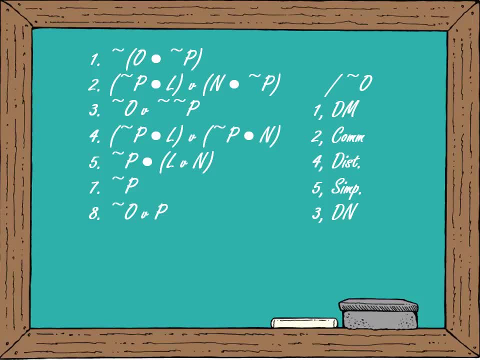 use double negation in order to get the tilde tilde p turned into a p And then switch by commutation to set up p in a position where premise seven can be used to help us obtain tilde o, which is our conclusion. 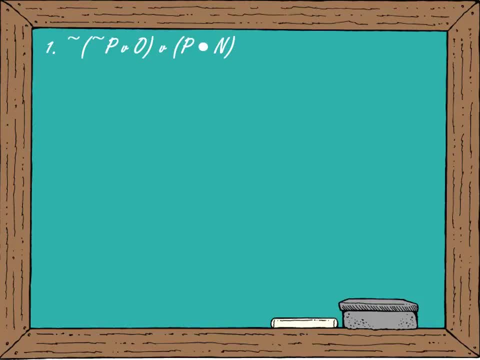 Let's try another example. How about this? A very long disjunctive premise followed by a simple one. The p implies o. The conclusion here is going to be n. Notice n is locked up there in that first premise. We need to. 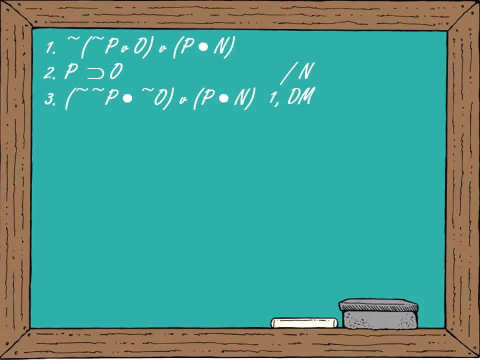 to take that first premise apart, first thing I always do is Dave Morgan's, when I can, in order to get the tilde within the parentheses, makes things simpler, and then by double negation: well, that's a pretty simple move on three. now what the reason why I did that? you can see, I was setting myself up for distribution. 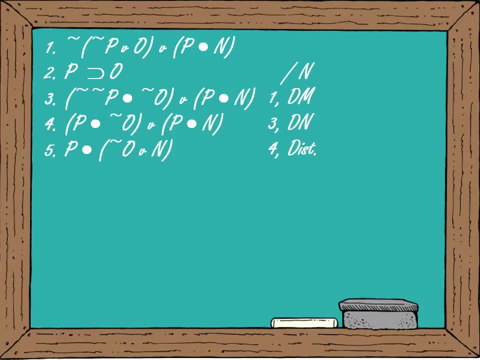 anytime that I can simplify a wedge claim like four down to a dot claim like five, I'm in a good position. then it can get out of, then I get a simple proposition P. I use that with, along with premise two to get to O. now notice, I'm setting myself up for a disjunctive syllogism in order to get to n, basically. 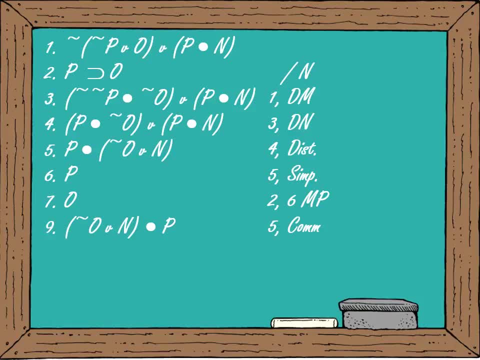 what I need to do is use commutative to get to that tilde o wedge n claim. once I do that and unlock it with simplification on line 9, then I can set myself up through double negation to do a disjunctive syllogism and I'm home. 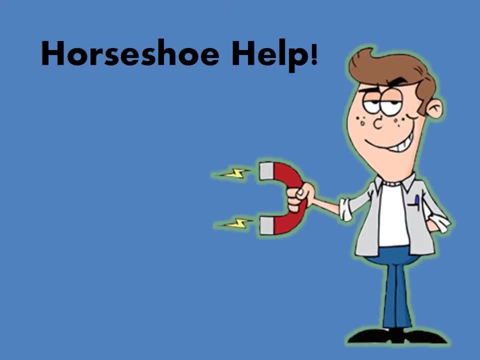 free. so far, we haven't had any rules to help us with conditional claims, so now I'm going to introduce two, because horseshoes are very important in logic. we're going to introduce two rules: transposition and material implication. you're going to use these an awful lot. 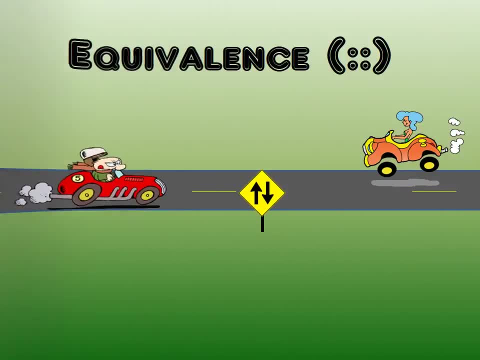 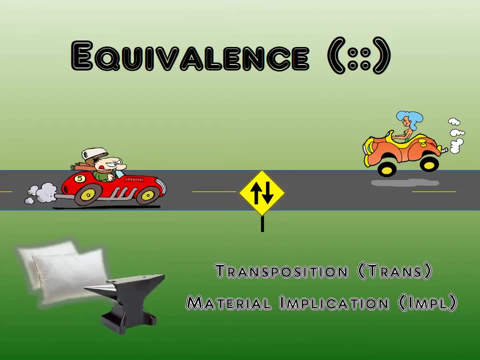 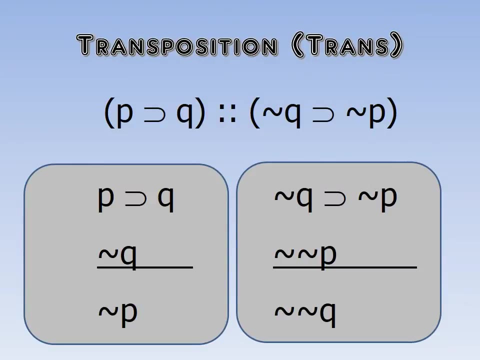 when it comes to dealing with conditional sentences- and again we're dealing with equivalence claims. transposition, I think, is a bit of an easy rule to grasp. material implication a bit harder now. regarding transposition, we said that when it comes to dots and wedges, you can switch the position of 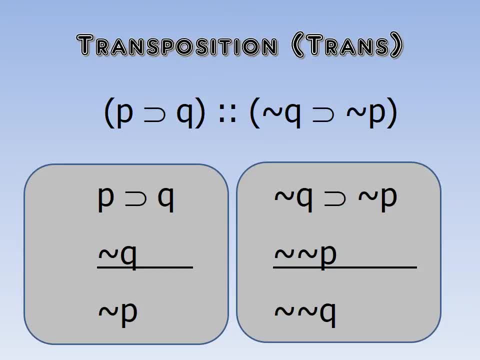 disjuncts and conjuncts, but you can't switch the positions of P's and Q's in this case around a horseshoe. it just doesn't work. but you can do that if you add another step where you negate each of the propositions involved. why does that work? 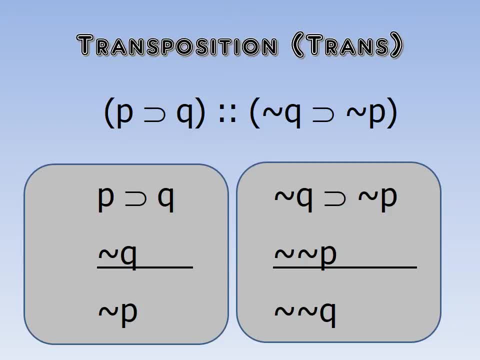 take a look at the bottom examples, where I have two instances of modus tollens. we began in the first premise around the first argument to your left with P implies Q tilde. Q, therefore, will take you to P. notice, that's pretty much just transposition, moving from the first argument to the second argument, to the 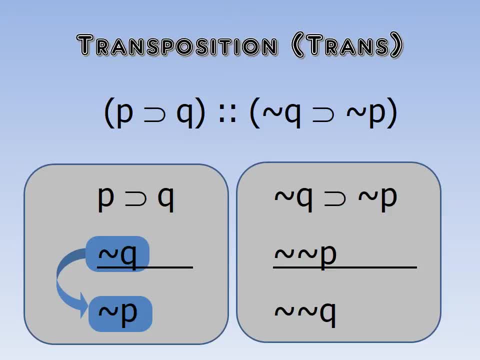 left formula to the right formula thereof. or look at the example to your right in the gray: tilde Q implies tilde P. wasn't that enough to say that double tilde P will take you to double Q, which is equivalent to the claim that P takes? 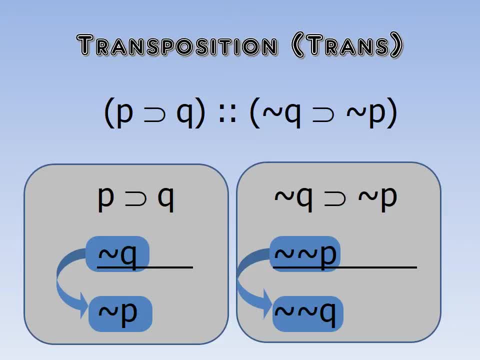 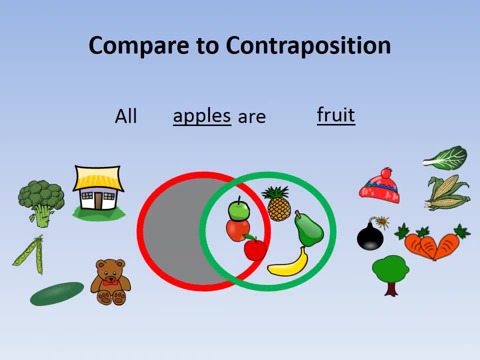 you to Q. that's why transposition works. it's basically an application of modus tollens simplified. compare this to contraposition. if all apples are fruit, we said, then if it's not a fruit, it's not an apple. well, if we said all bulls are cows, then basically what that means is that all 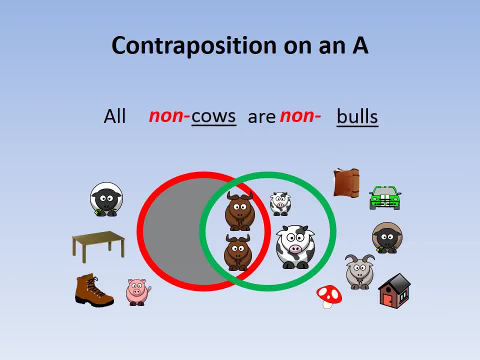 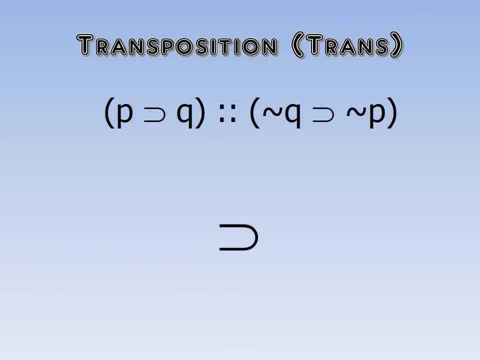 the bulls are in the cow class and consequently that if it's not a cow then it's not a bull. well, if you recall how contraposition works, transposition to be easy to remember. basically, in the case of propositions, the proposition it's an apple implies it's a fruit. true, we can't just commute the two propositions and 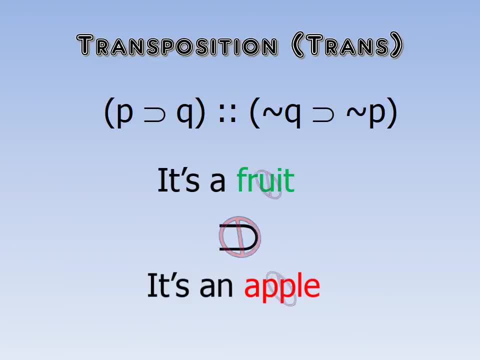 it's a fruit does not imply, of course, that it's an apple, but that if it's not a fruit, that certainly implies that it's not an apple. again, switch the positions and negate. now you can use this in a variety of ways, for example, just flip. 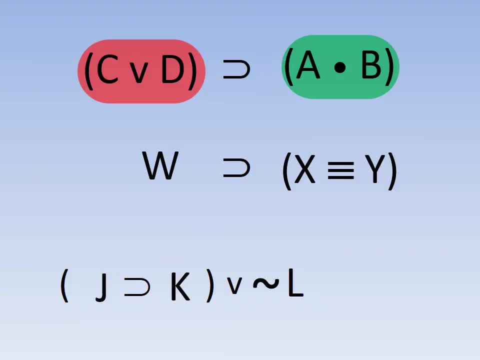 flop the two complex propositions around a horseshoe, add your negatives. we just did it with more complex propositions. or in this case, flip, negate, the move works again. or in this case, we can use it on part of a proposition, since it is a rule of equivalence. so we'll just take the two propositions, move them into. 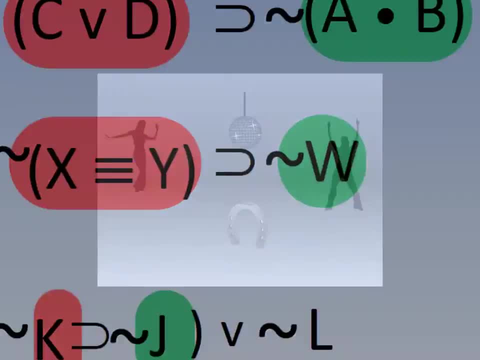 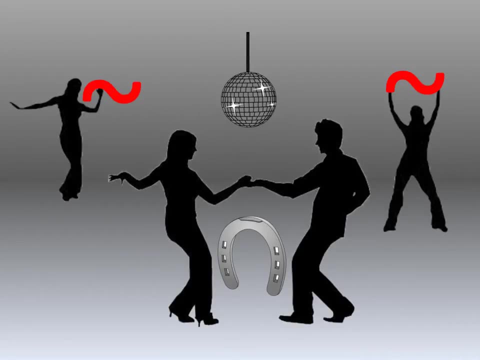 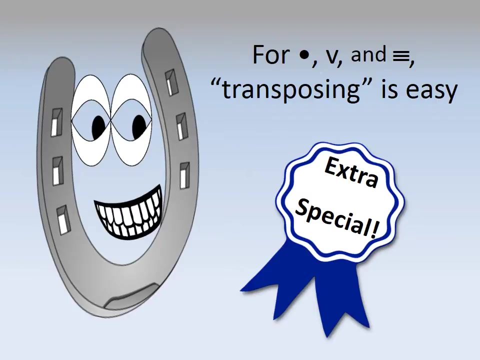 different positions on the horseshoes and negate. so remember, do all the spinning of your propositions around the horseshoe you want. just remember to bring those negatives with you. now for dots, wedges, and in a moment we'll see biconditionals. transposing is easy. 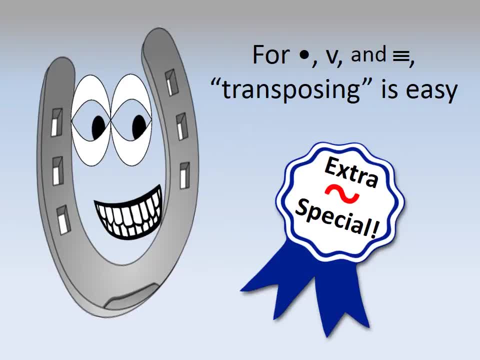 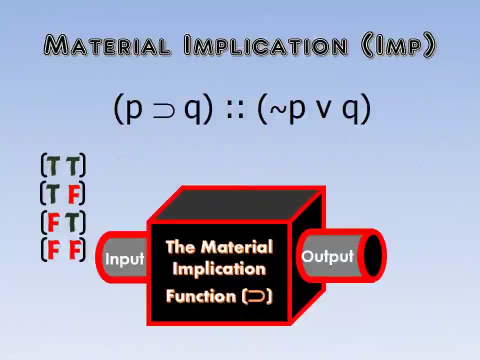 just flip flop the two propositions. the horseshoe is extra special. bring along your two tildes and you'll do okay. the second rule that we have for dealing with horseshoe claims is the material implication rule, dealing with the material conditional we have to remember. 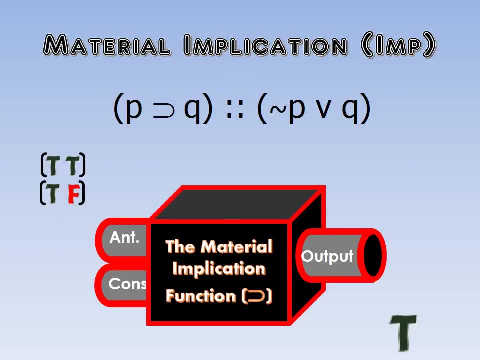 that what goes in the antecedent and consequent columns makes a big difference and we only get an output of false right there, where the antecedent was true and the consequent false. now, if you can remember this truth table for the horseshoe, then you should be able to remember the material implication. 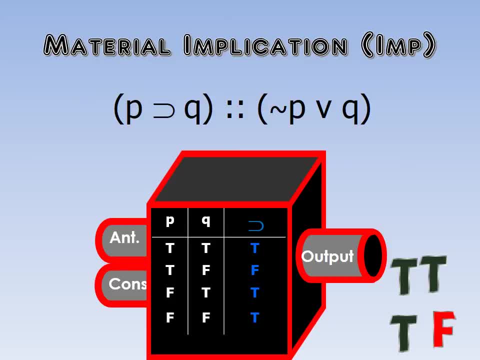 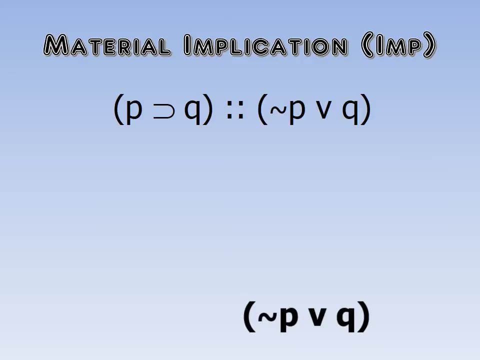 rule. this table should remind you that all the horseshoe claims is that you're not going to get, or rather that you're going to get either a false antecedent or else a true consequence. but for those who like a actually a formal demonstration of the equivalence of these two claims, let's go ahead and take. 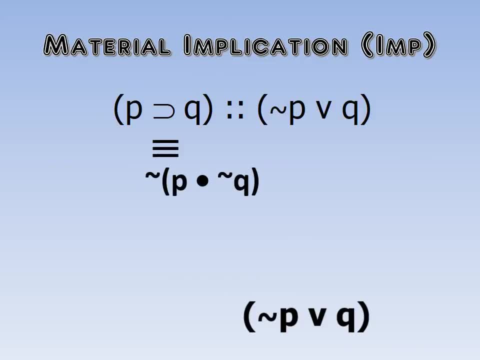 a look now we know that P implies Q is pretty well equivalent to the claim, that it's not the case that P and tilde Q, not the case that true antecedent and false consequent. that's what the table told us right now. if that's the case, then, that a claim is also equivalent to. 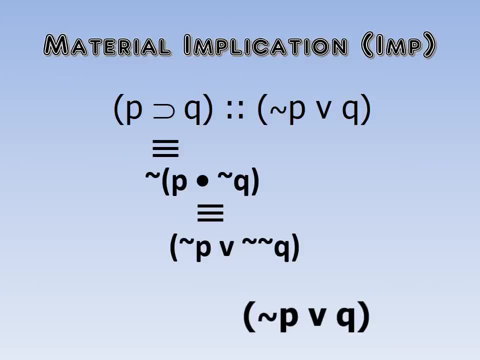 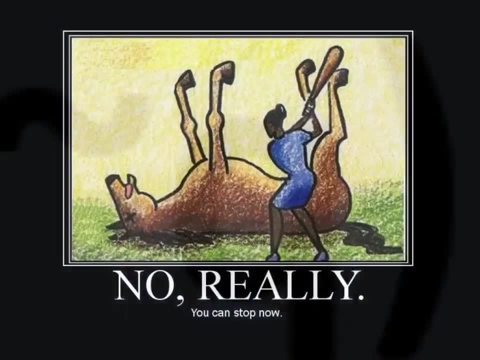 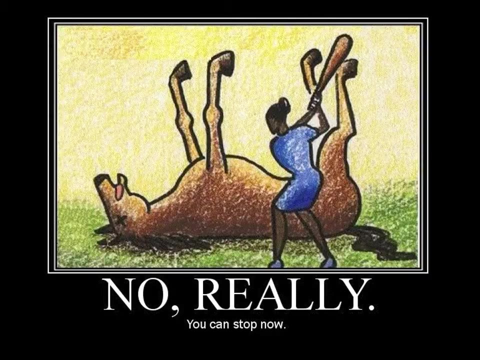 the claim that by De Morgan's rule, tilde P or else tilde tilde Q, and by double negation- yep, you got it straight to the bottom. okay, enough with the formal demonstrations- is exactly why material implication works by and large. I guess you're just gonna have to memorize the rule. but you're gonna have to memorize the rule by and large. I guess you're just gonna have to memorize the rule. but. 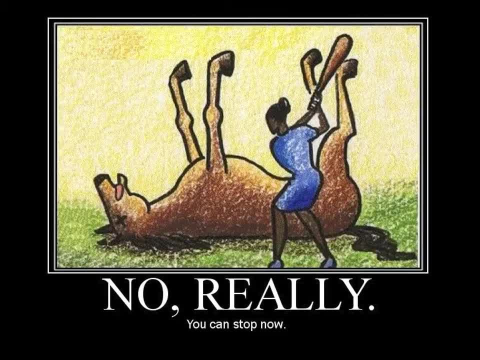 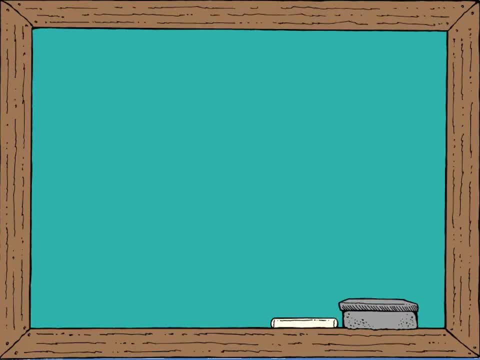 if you know your truth, table and formal proofs of how material implication is derived. I think you're a long way towards understanding and using the rule, let's try to do a proof in which we have to deal with a lot of horseshoes. tilde H. 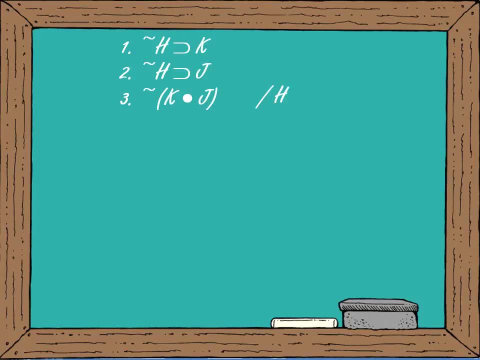 implies K, it also implies J, and it can't be the case that both K and J. now, that third premise should tell you that if it can't be the case that both of them, then we should be able to do modus tollens or something like that, on either one or two. 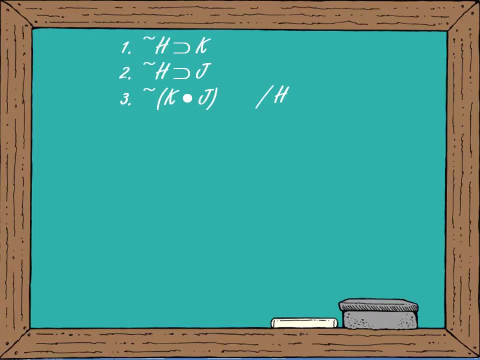 and get to our conclusion H somehow. But we're going to have to do a lot of work with horseshoes to get there. First things first. I want to do De Morgans to get that tilde distributed. I don't like tildes. 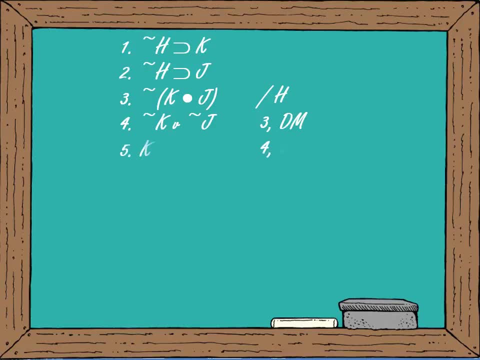 in front of parentheses as a general rule. Now I'm going to do implication to get a horseshoe claim out of this. By line 8 in this proof you're going to see why I just did that. What I'm going to try and do is say that tilde H implies tilde J by hypothetical. 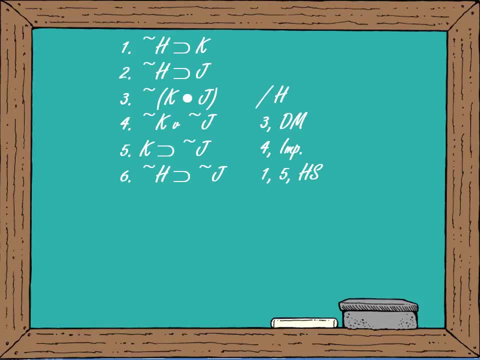 syllogism. Look at lines 1 through 5, where K does the linking up work, Then J implies H by transposition. I just took line 6, flip-flopped and dropped the negatives. Now doing that? 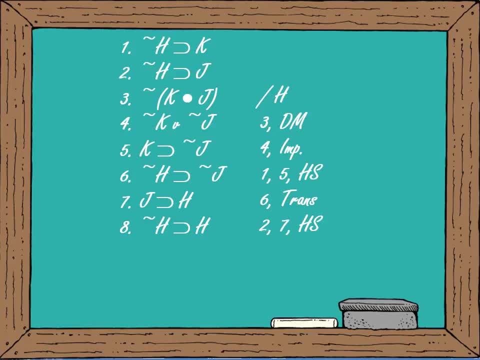 I can do hypothetical syllogism one more time, this time using lines 2 and 7. I told you by line 8 you'd see what I was up to. Line 8 shows you a little technique that's very important in proofs. If anything implies it's opposite, then that opposite is going to be. 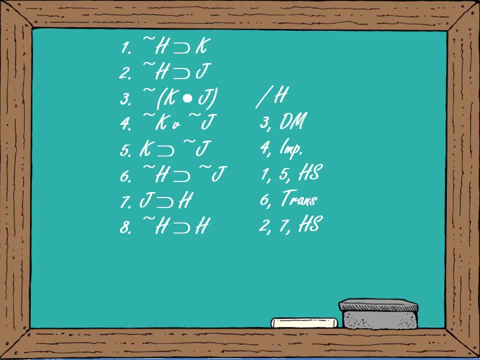 true. How do you know that This trick always works? It will get me to H or the consequent every time. All you've got to do is use implication. See the importance of the rule there. Once I drop that double negative that I have in 9, I get H or H, and I told you this rule. 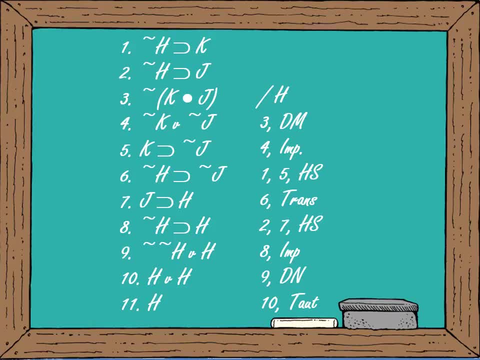 would be useful. by tautology Now you can tell why I tried to get to line 8.. Any time I get a claim like that, there's a little trick, like lines 9 through 11, that will always get you to the truth of the consequent, like in 8.. 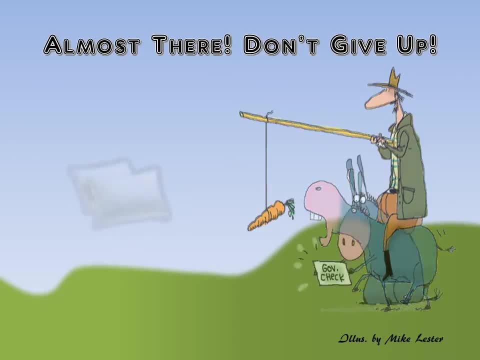 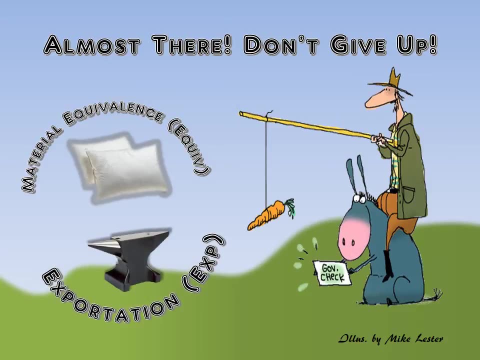 Okay, I know you guys must be getting tired. Please don't give up. I've got a little trick here. I'm going to show you a simple rule- material equivalence- and one that's a little difficult. Let's take the easy one first. The first rule is going to deal with 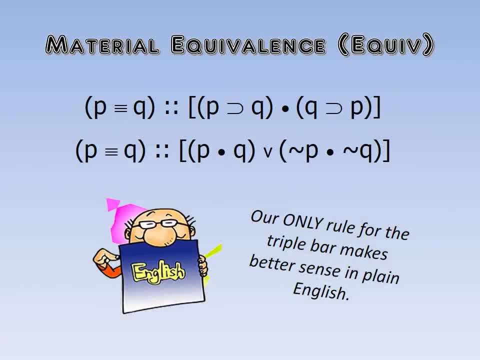 biconditionals. Material equivalence is the only rule we have for dealing with triple bars and it's the only rule for triple bars you're ever going to need. The first version says that if P triple bars to Q, then P implies Q and Q implies P. The second version: 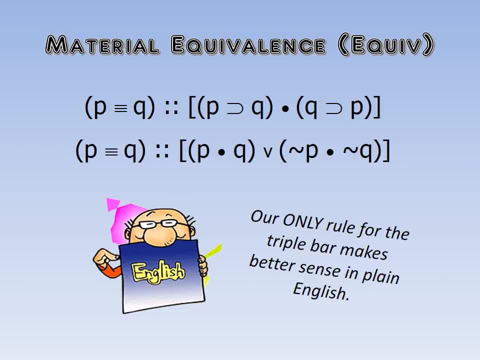 says that if P triple bars to Q, either P and Q are both true or P and Q are both false. Notice: these rules make better sense when we put them in plain English. It's what you've known about the triple bar all along. only here we have it laid out in explicit, formal terms, and it may be. 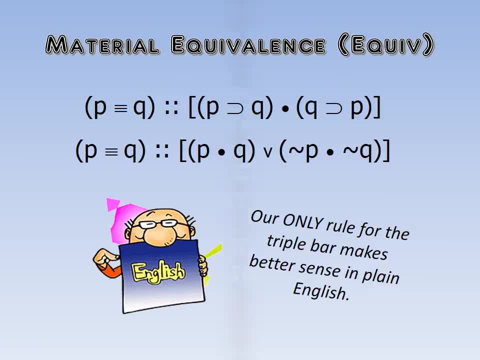 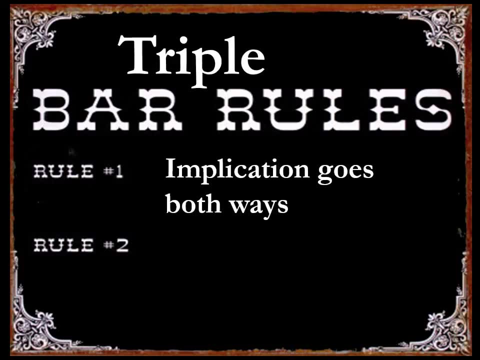 a little difficult to read. Read it a couple times and you'll get the basic concept. The basic concept, basically, well, goes like this: The triple bar rules. state rule number one. implication goes both ways and if a triple bar holds, either both propositions are true or both are false. 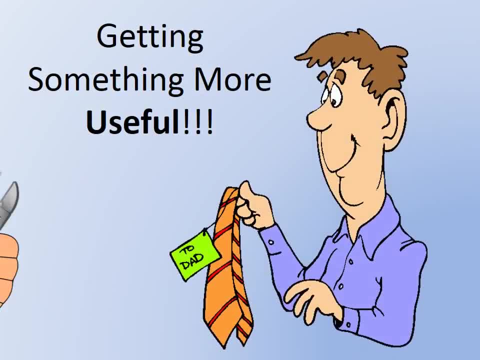 Just that simple. Now. the triple bar rule, or material equivalence, is really helpful when you need to get something more useful. Let me give you a couple instances of this. Here's a couple of useful tricks when you're using this rule. Look over to your left. If p triple bars to q, does q. 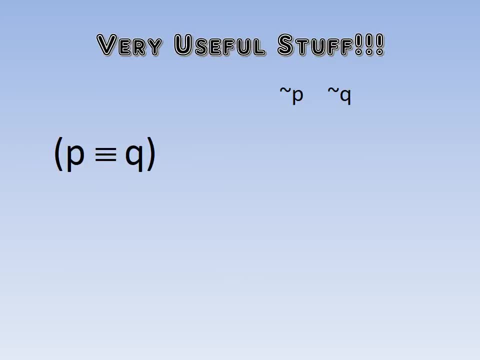 triple bar to p. We didn't have a rule of commutivity for the triple bar, but the rule that we have will give you that, because what our rule says is that what this triple bar amounts to is p implies q and q implies p. So if you're using this rule, you're going to have a rule that you 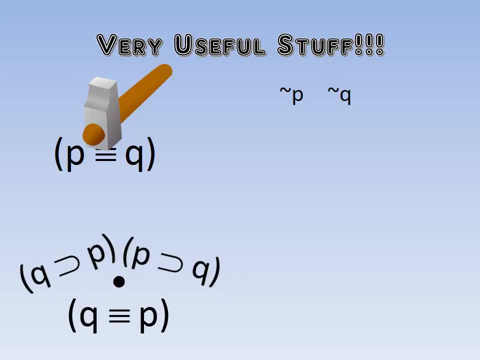 can commute around the dot and therefore arrive at the claim that q does triple bar to p. So in this extended sense, yes, we do have a commutivity rule for the triple bar thanks to material equivalence. Now look over to your right. Suppose you find out that p and q have the same truth. 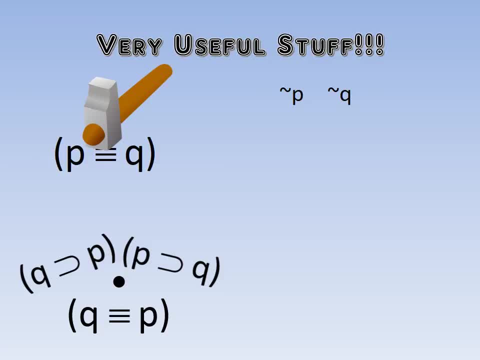 value, namely tilde p and tilde q. Can you get a triple bar out of that? Here's a trick: Just go ahead and conjoin the two lines that you have and form one conjunction through a conjunction and then, because you can conjoin and then wedge off to any claim you want, just wedge off to pq or. 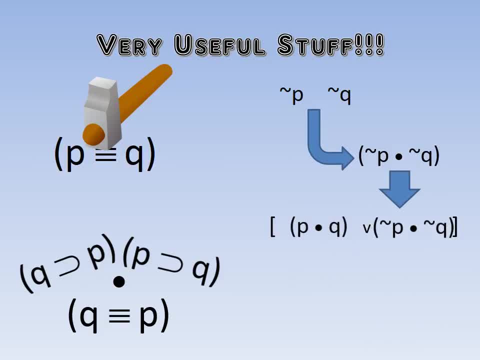 anything else for that matter, you can commute around a wedge. So through our triple bar rule, this is equivalent to p implies q. This is a trick that you can use any time that you know propositions have the same truth value to get a triple bar out of it, Useful in many proofs. 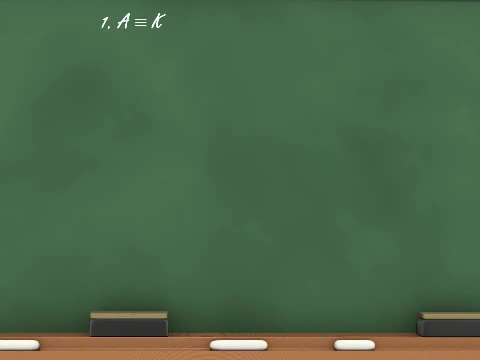 So let's use a proof where we have to use our triple bar rule thanks to premise number one here, and we'll have a disjunctive premise of tilde a or tilde k, and r implies a. Does it follow? 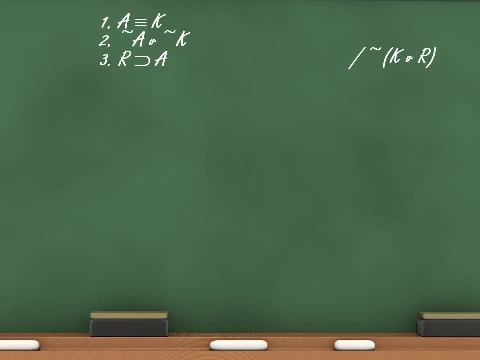 that tilde k or r. Now here I want to show you another trick with respect to proofs. Look at that conclusion. That's a little bit too hard to derive all by itself. I'm going to give away a hint. If 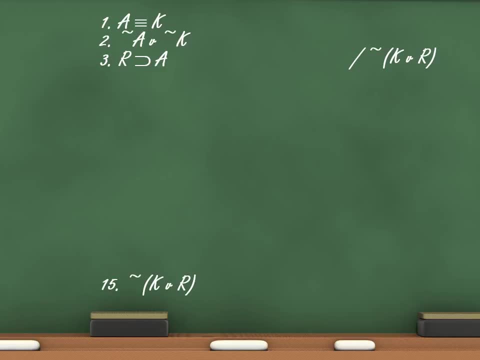 we want to derive, by line 15 of our proof, the conclusion in question. we need to reach it through double negate, or rather De Morgan's rule. What we need is to get to line 14.. From our premises I suggest we try to prove tilde k. 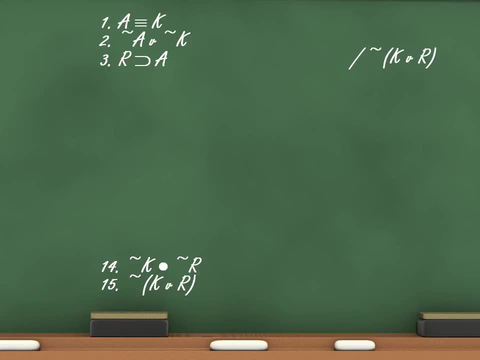 and then we try to prove tilde r. then we'll conjoin them by line 14, and then use De Morgan's rule to get to our conclusion in line 15.. That's a good strategy, I think. First step we're going. 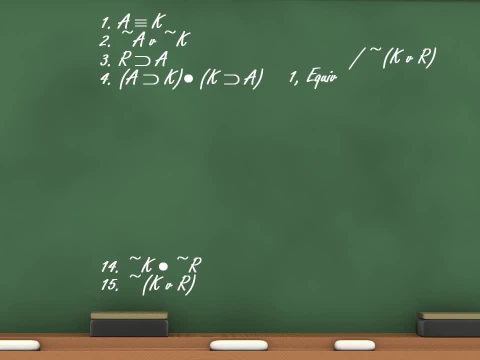 to do is use the equivalence claim that we just studied to dismantle premise number one. And since I think I want to deal with k horseshoes to a first, I'm going to just flip-flop those two by commutivity so that I can simplify down to the first conjunct in five Once I've done that. 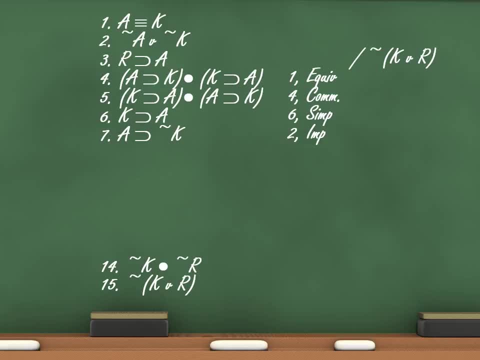 I'm going to use implication on line two, because I don't like to deal with wedges, I like dealing with horseshoes better. Notice, that sets me up for a hypothetical syllogism. Now, if you remember our last proof, you can tell right away. 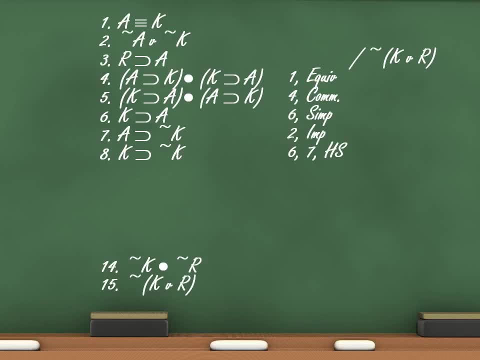 why I wanted to get to line eight In a few simple steps. I should be able to prove from this sort of line that tilde k is the case. I do that by the same moves as before. Implication to tautology. 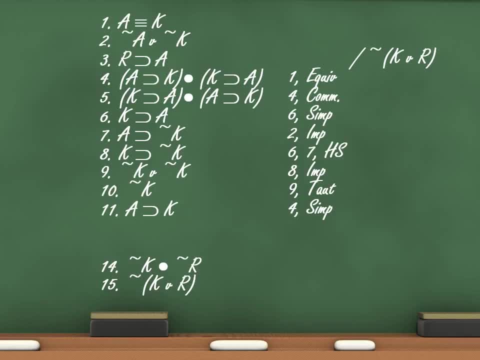 There we go. We're halfway there. The next step: I'm going to do a simplification on line number four and get to A implies K, sort of like. I simplified 5 before I'm going to get to line 12 by modus tollens. 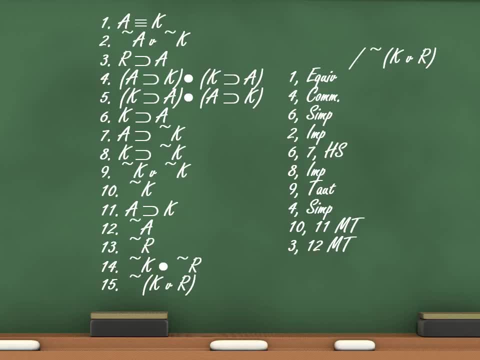 Line 10 is helpful there, And then 3 and 12. modus tollens is going to give us the second conjunct that we need. Line 14 follows by a simple conjunction and De Morgan's rule gives us our conclusion. End of proof. 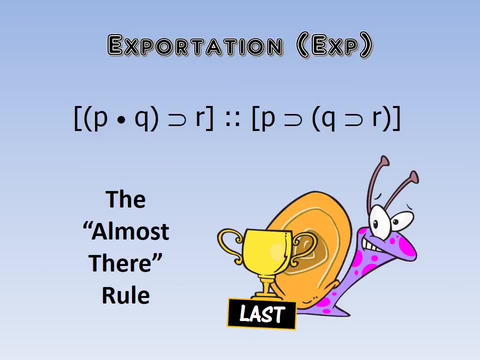 And it's almost the end of our lectures on these new rules. Because exportation- I promised you would be a hard rule to learn. P and Q together imply R is basically the equivalent of saying P implies that Q is enough to get you to R. 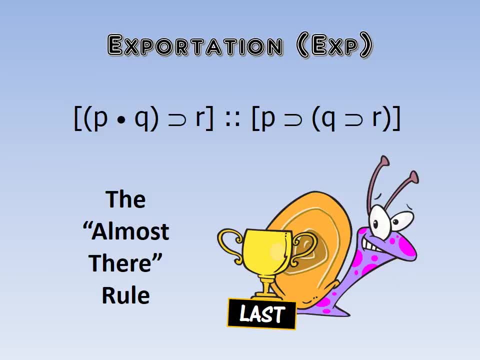 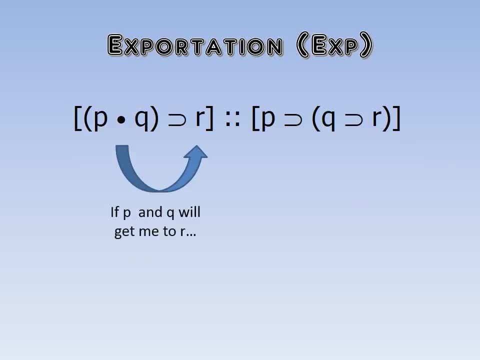 Well, how does that work? I call it the you're almost there rule. Here's how I'll explain the rule to try and make it more intuitive. Basically, what this rule says is that if P and Q together will get me R, then that means that if you have P already, then Q is the last thing you need, and Q will get you there. 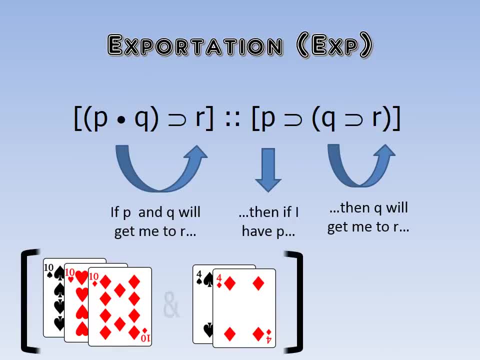 Here's an illustration. Suppose somebody says if you have three 10s and two 4s together, that's enough to get you a full house in a card game. Well, what that is equivalent to saying is that if you already have three 10s, 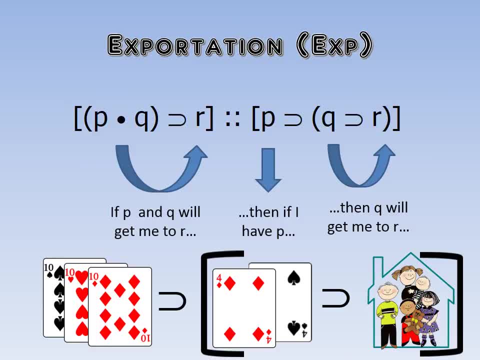 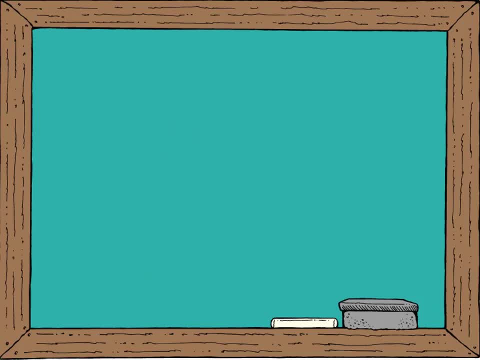 well, then that implies that you're almost there. All you have left over is to get those two 4s, and then that will get you a full house. It's basically, you're almost there. Here's a short illustration of how to use the rule. 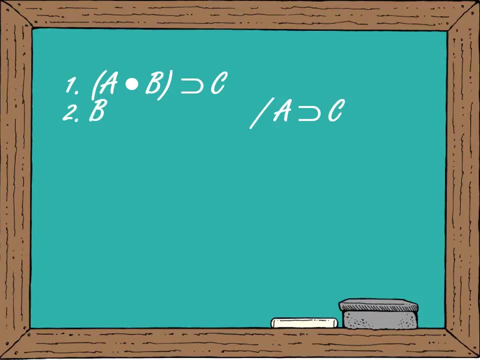 If A and B together imply C and you've already got B, well, it looks like you're almost there. All you need left over. All you need left over is A to get to C, as the conclusion says. This conclusion should follow. 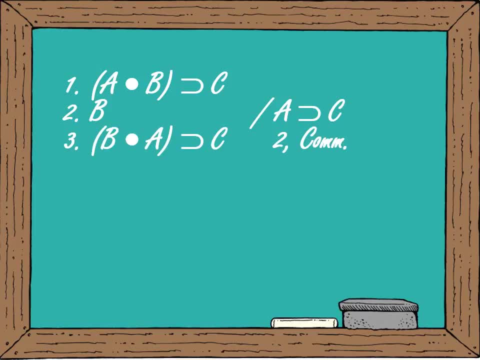 We need our exportation rule to show us why. First I'm going to commute B and A so that we get B right out there in the front, and then I'm going to use exportation. By exportation, B implies that A is enough to get you to C. 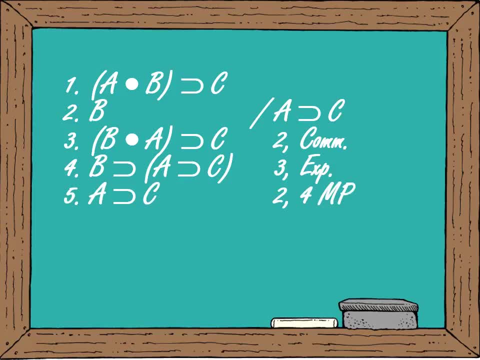 Notice what I did. I set us up for modus ponens with line 2.. A really is enough to get you to C, given line 2 that one of the conditions for C has already been met, You just have another one left over. 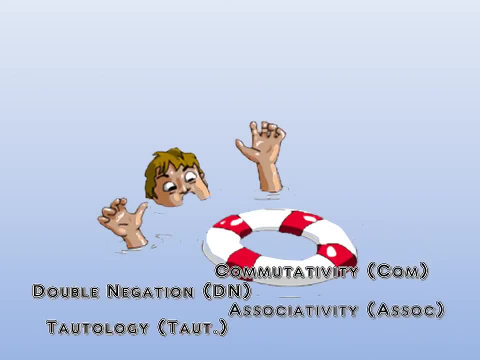 Now you might feel like you're drowning in all these rules. It's going to take a little while to get your mind around all of them. no doubt They are kind of difficult. This is going to be one of the most difficult lessons that you've had. 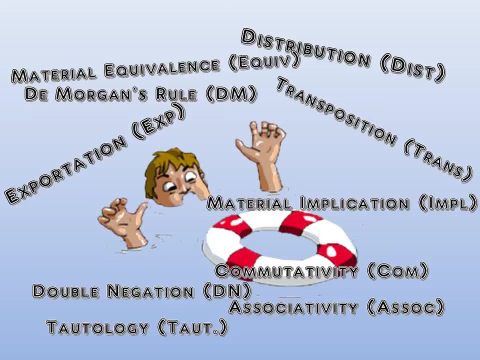 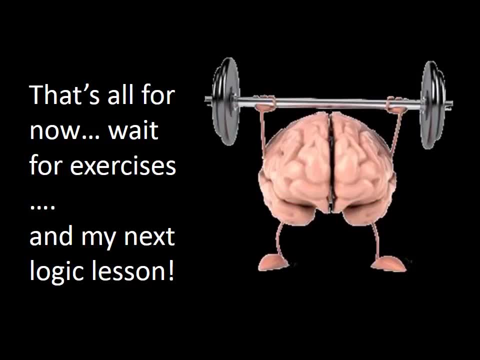 I'm going to provide a lot to help you later to get your mind around these concepts even better. So plenty of exercises to come. They're going to be necessary in order to wrap your mind around the concepts you've just studied. In the meantime, watch this video a few times. 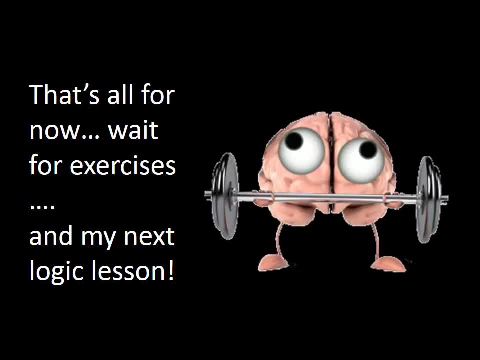 and hopefully you'll have a lot of fun with your logic textbooks. Take care, and we'll see you next time for our very last lesson in this first lecture series on logic.